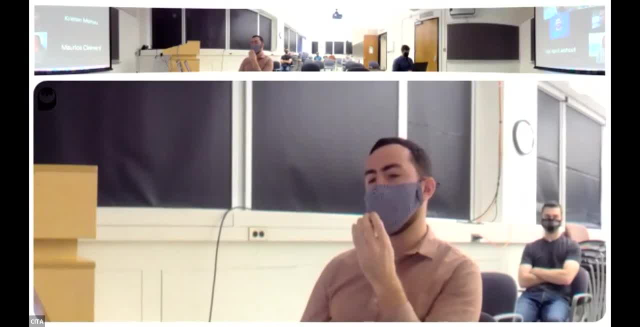 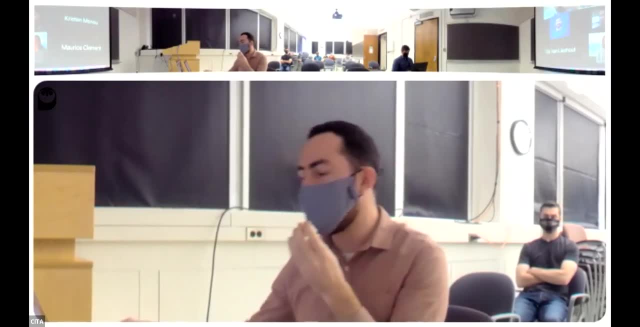 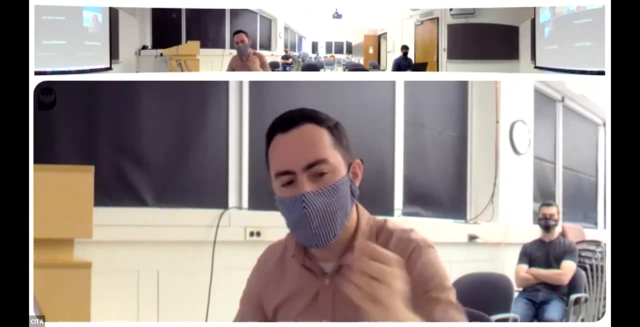 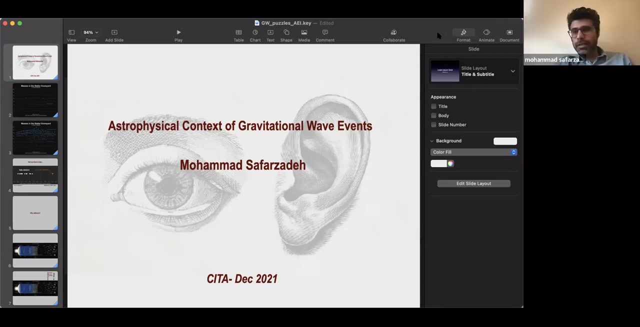 Astrophysics at UC Santa Cruz and Arizona State University. He did his PhD at Johns Hopkins in 2016.. And today he will be speaking about the astrophysical context of gravitational wave events. So, Mohamed, whenever you're ready, please take it away. Okay, you see my screen. 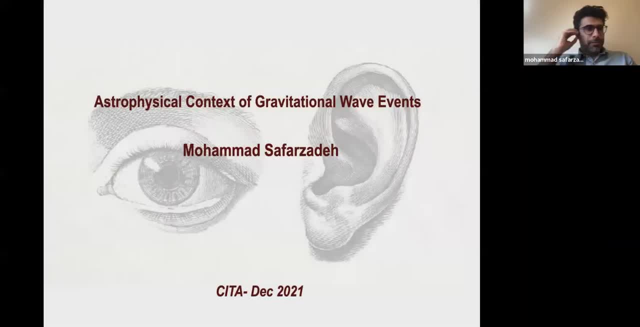 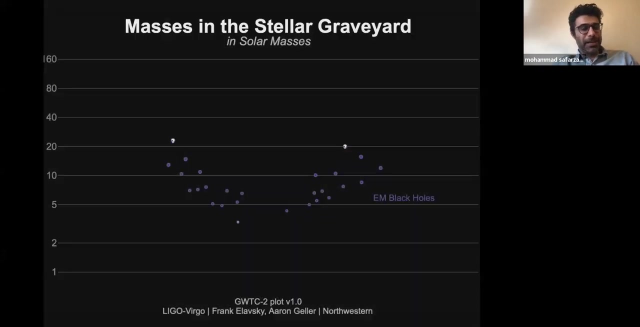 Yeah, Okay, Thank you very much for the invitation, And I was planning to speak about a completely different topic, But today I'm going to talk about what I've been working in the past year or two, And I'll start with a deep dive into the core question. The question we are trying to address is the 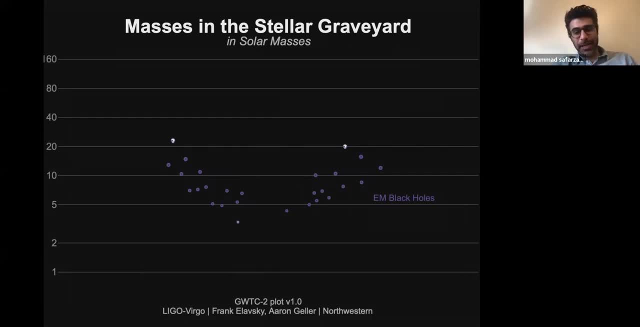 difference between the black holes that are discovered through electromagnetic waves and those that LIGO and Virgo collaboration find. So if you look at the mass distribution of black holes detected prior to gravitational wave events, we see that most of them range from between five to almost 20 solar masses. However, in gravitational waves, when we look at the sky through, 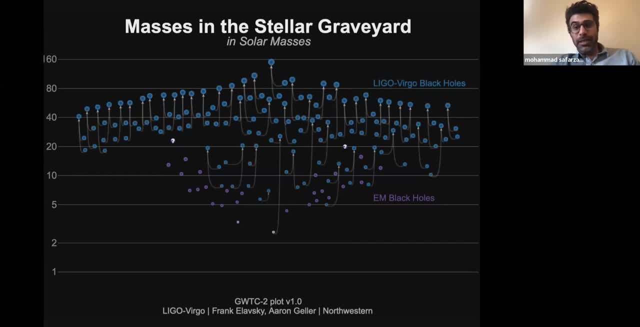 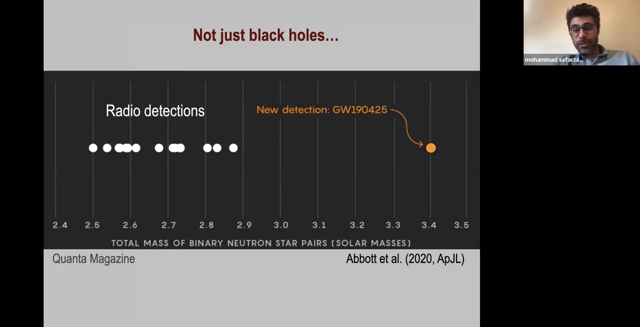 gravitational waves, we see a wider distribution and definitely more massive black holes have been discovered since, And this is not just black holes, It's also neutron stars. For example, we have a detection of 190425,, which is a binary neutron star with a total mass of 3.4 solar mass. 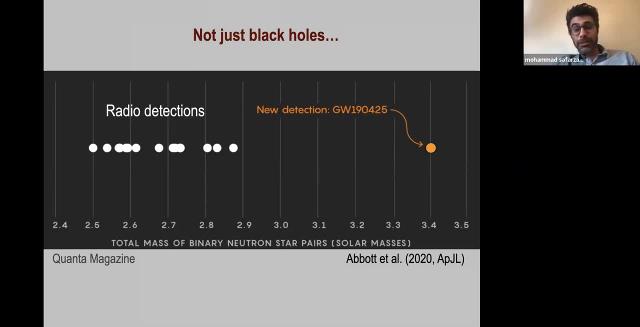 And, however, this is tensed about more than three sigma away from the distribution of total mass of binary neutron star systems that are found in electromagnetic observations. Now the question is, why is there a mass difference? And if you step back a little bit, you 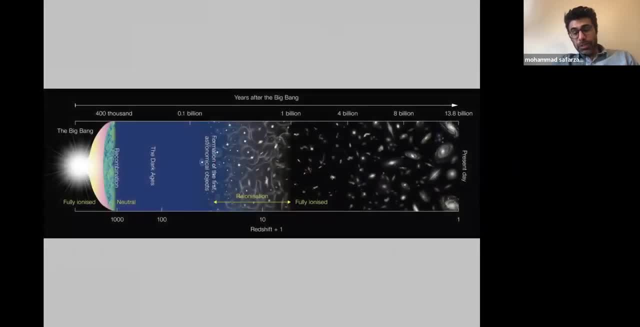 can see a relationship is very good. For example, the mass is the same, but the material distribution of the speakers of a galaxy and another mass is different, And that's where we will likely want to learn more about the mass distribution. We want to know what the mass distribution is going to be. 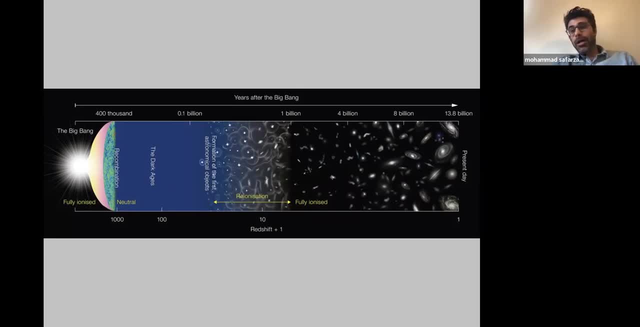 and we can use it to find out what's happening in the universe in these changes. So the question is: how do we, Может we know what's going on in the universe in these changes? We can, uh, we can look at the uh, just how the universe has been evolving from Big Bang. we know. 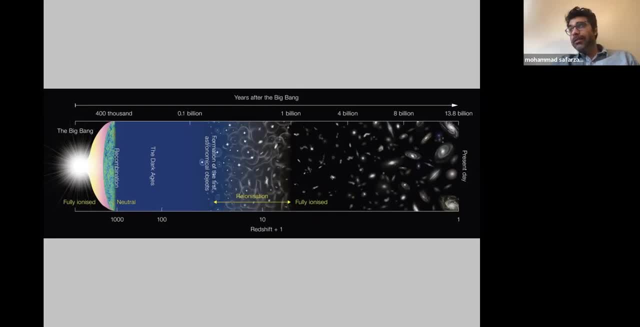 that stars in the structure has been forming very high red shifts And this has been going on through a hierarchical structure formation. and the hierarchical starship formation matters because, well, first, we know that what we are observing currently, we have been observing a gradation of the galaxy And we have been improving the galaxy National tiredness. 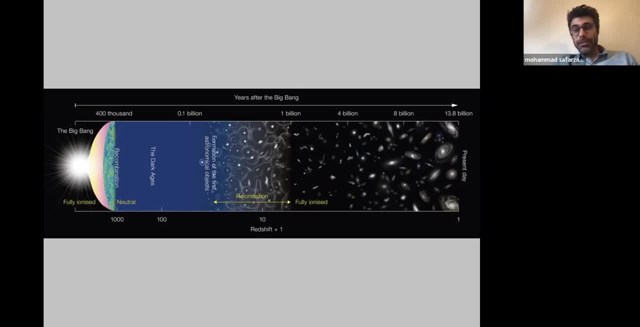 what we are observing currently by gravitational wave detectors are all the systems that merge in the local universe. So the first question is: when did these systems form that they merge now? Is there a short delay time between their formation and merger, Or is there a long delay time? 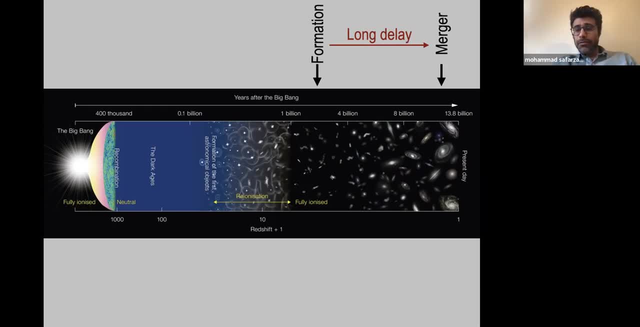 And this matters because through hierarchical structure formation, we know that the universe becomes more and more metal-enriched through the ejection of metals through supernovae, And we know that also at high metallicities, stars lose a lot of mass through their winds. 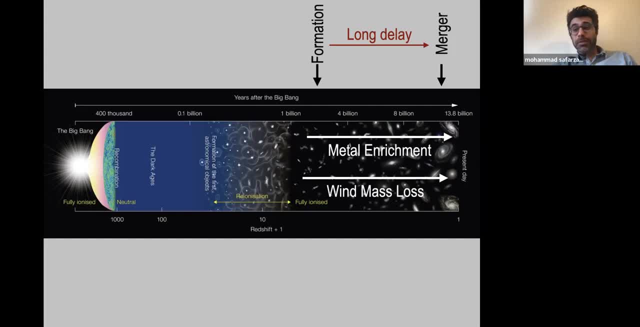 So a star of a given mass at two different metallicities will leave behind two different black holes after the supernova explosion. The more metal-enriched, the more metal-enriched, the more metal-enriched one will leave behind a less massive black hole. 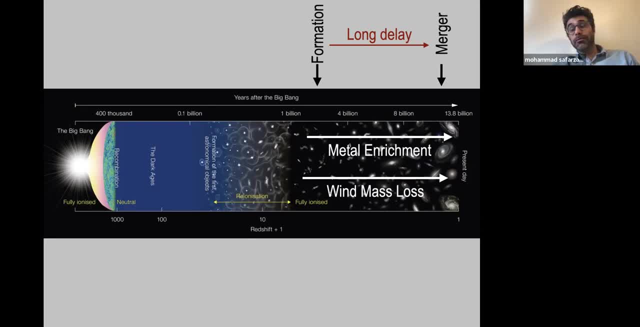 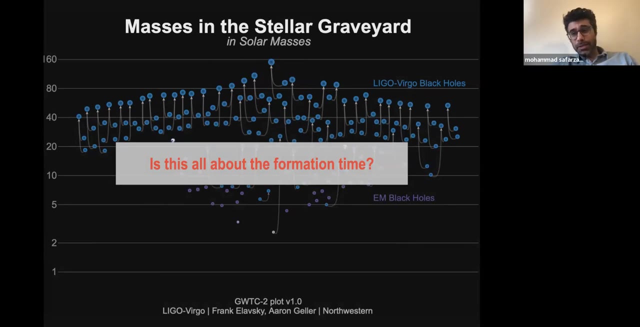 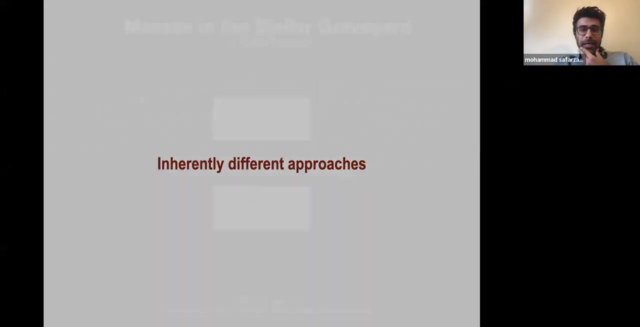 because the star has lost most of its mass through wind loss at higher metallicities. So it's a little bit complicated And the question here is whether this whole difference that we see is it all about the formation time. There are different approaches that one can adapt. 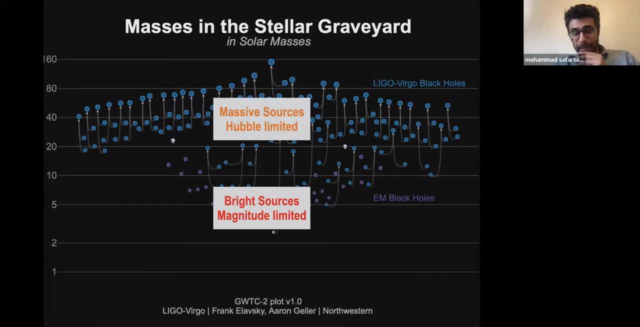 However, one should be aware of the fact that- and this is a very important point- one should be careful about some biases that we have. We know, for example, electromagnetic discoveries are always limited by the brightness of a source, And we are always- our surveys are always- magnitude limited. 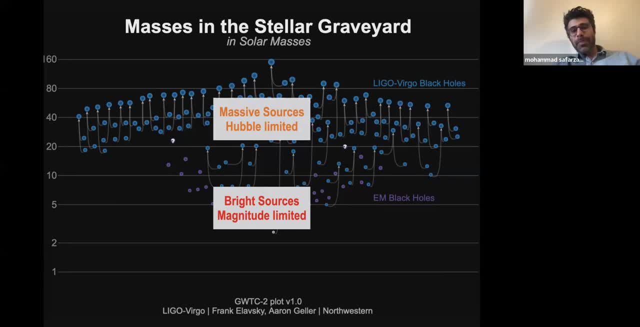 However, the gravitational wave approach has different limitation in terms of the mass of the source. We are limited by the mass And we are Hubble limited in the sense that we only see systems that merge within Hubble time. So these are important constraints. 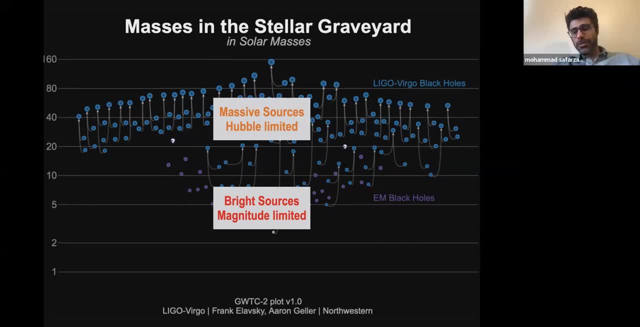 So that we have to always remember when we want to have an interpretation of systems we observe. Moreover, we know that the gravitational waves are all sky surveys And, unlike our deep surveys and electromagnetic waves, that we can pinpoint the position of the sky and do a long integrated observations. 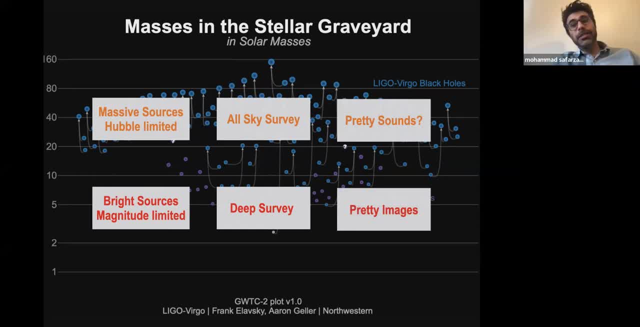 And what we have in electromagnetic waves are basically pretty sounds because the at the moment our observation, our observation of gravitational waves fall into human audible range. But on the other hand, we have basically pretty images When we look at the sky through electromagnetic waves. 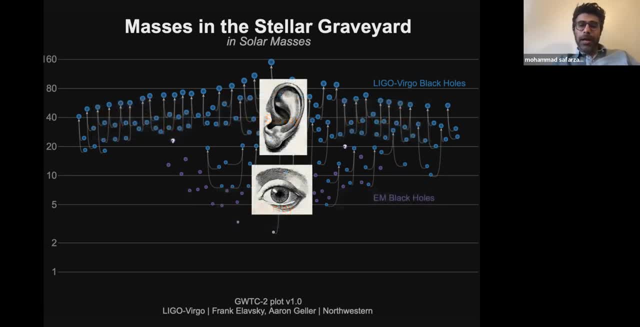 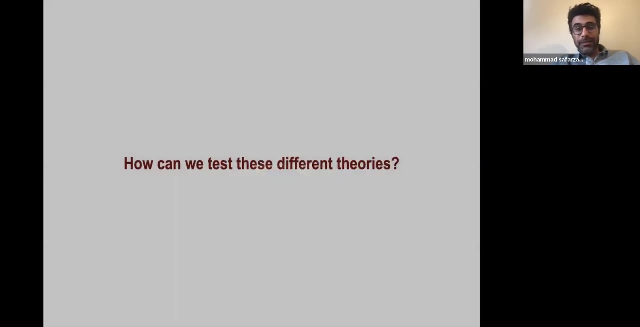 And this reminds me that perhaps it's better to see, to say that the universe as we listen to is different than the universe as we see, And I will say that, okay, now we want to test different theories about the formation and what is the best way to proceed. 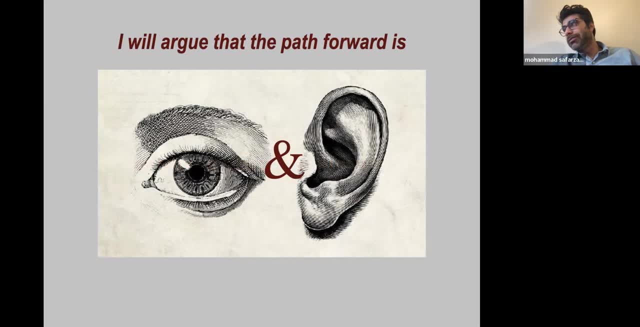 And I will always. the point of this talk is that I will, I will argue: you have to combine both knowledge, both approaches to get the holistic picture of what is going on in nature, basically. Otherwise we're going to have a biased interpretation. 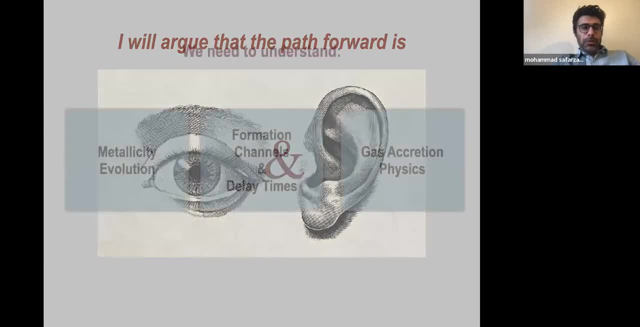 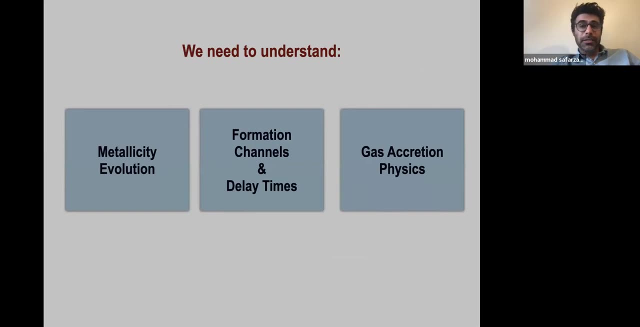 which is incorrect. So three things that we need to understand are metallicity evolution, formation channels and their delay times, and the physics of gas accretion. These things will impact. these are basic things that you have to understand in order to have a model. 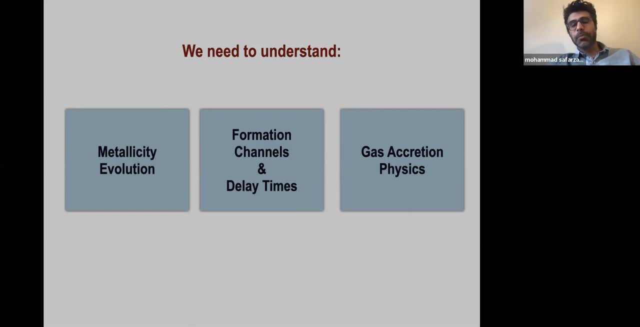 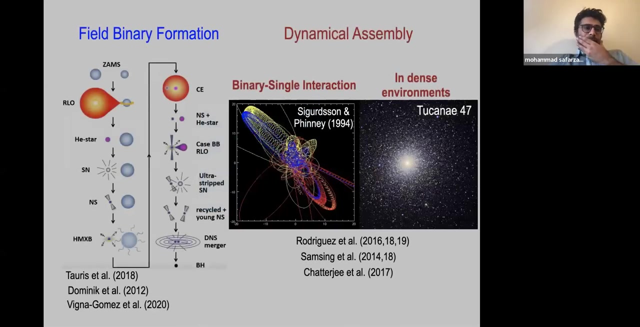 to predict the mass distribution of of compact objects that we see in gravitational waves. To start, I will focus on the formation channels and delete a very quick introduction and a small part of this talk. Broadly speaking, the formation channels are divided into field binary formation. 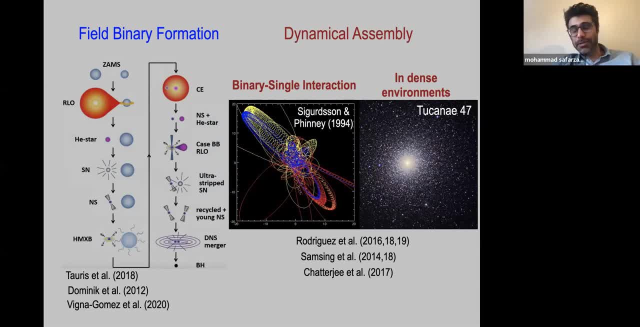 where two stars start from zero-h main sequence. two zero-h main sequence stars evolve through a so-called common envelope scenario, in which the stars lose their envelope and the distance between the two progenitor starts to shrink as a consequence, and then they become enough close. 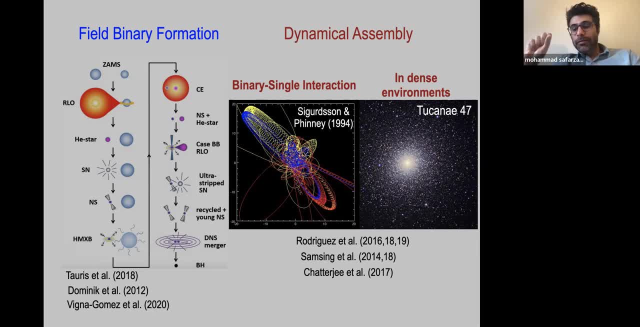 to each other, that after two supernova explosions are close enough to each other that they can merge within a Hubble time, And there is maybe thousands of papers on archive to read about different variations of this mechanism For different masses of binary compact objects. 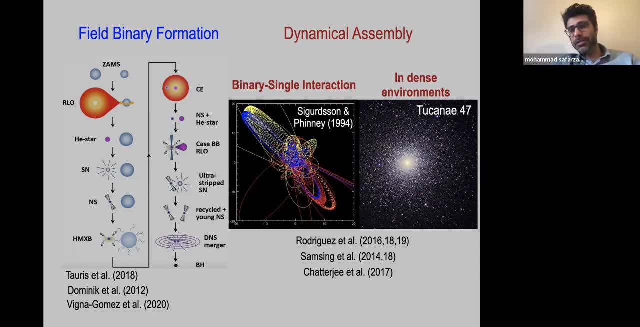 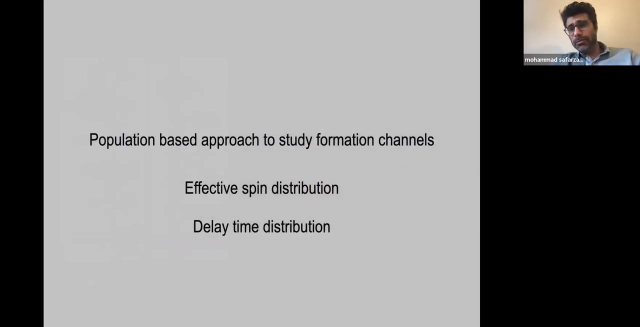 And the other scenario is, of course, the binary single interaction in dense environments, either in globular clusters or galactic nuclei, And different mechanisms have different predictions, of course, for the global statistics of compact objects, And one of the there's two ways that I will briefly talk about today. 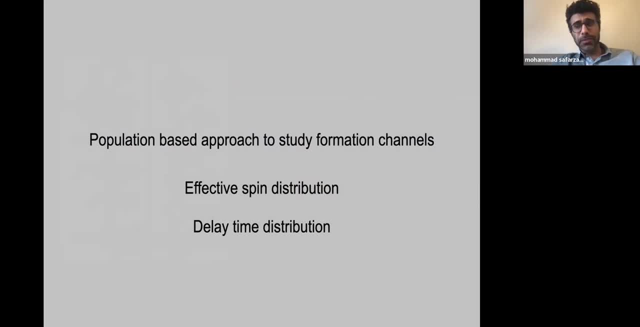 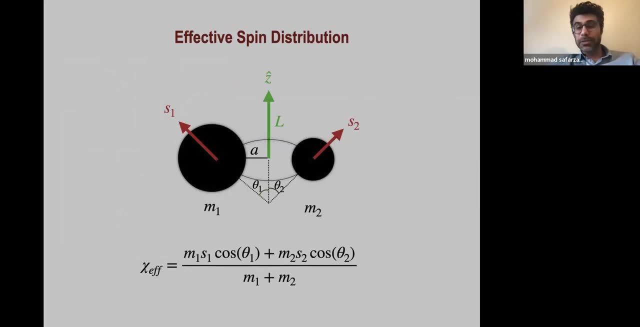 Are the studies in the effective spin distribution and delay time. distribution And effective spin refers to the projected spin angular momentum of the binaries onto the angular momentum vector of the binary, So it is a mass weighted. mass weighted spin projection of the compact objects in the binary. 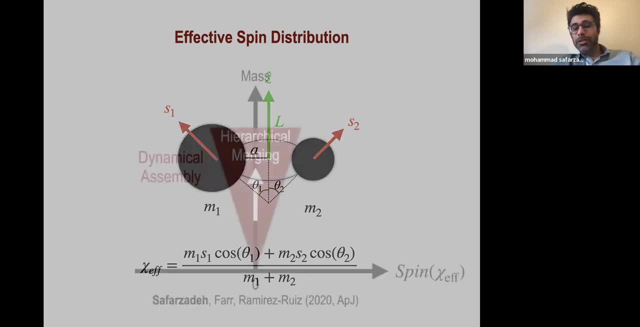 onto the angular momentum axis of the binary And different models predict different distribution. For example, in a dynamical assembly model in dense environments the two black holes come together with no regard to the spin orientation of the other one. So the expectation is that, as the hierarchical merger 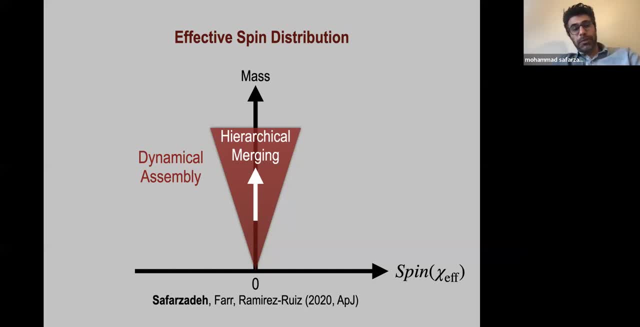 happens, the spin distributions remain symmetric around zero and grows with mass. That is the simple prediction of dynamical assembly. However, in field binary formation, it is expected that components of the binary will tend to be aligned with the angular momentum vector, And so different models predict either zero. 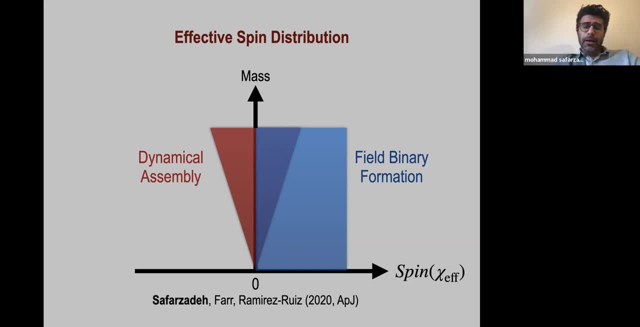 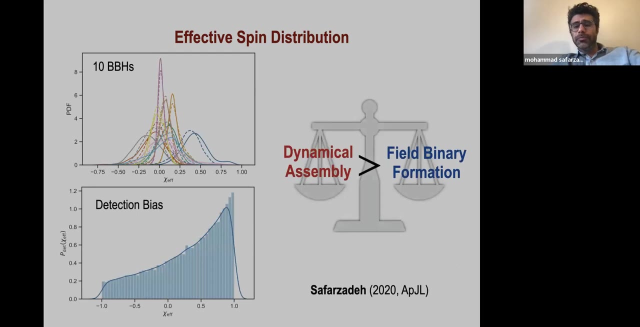 effective spin or positive effective spin. If we believe in this, It's a very simple first-order approximation, of course, of how these models predicted distribution in the spin. But if you adopt this, you can go back. This is a work that I did in the first 10 binary black holes. 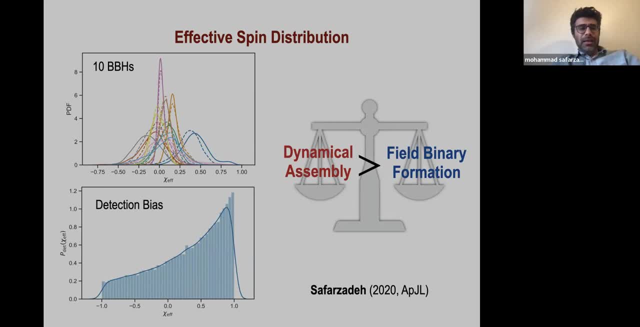 that was released early on in 01.. One can have a look at the distribution of effective spin of the black holes. So for each binary black hole there's a PDF of the effective spin- And by considering this and knowing the detection bias, 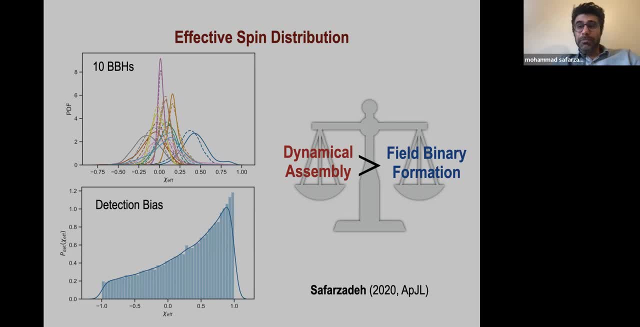 you can get a sense of whether there is a support for symmetric distribution or not. Basically, how much support do we have for negative effective spin or chi-effective? And what I concluded back then was that the spin distribution is not only a non-negligible, but it also 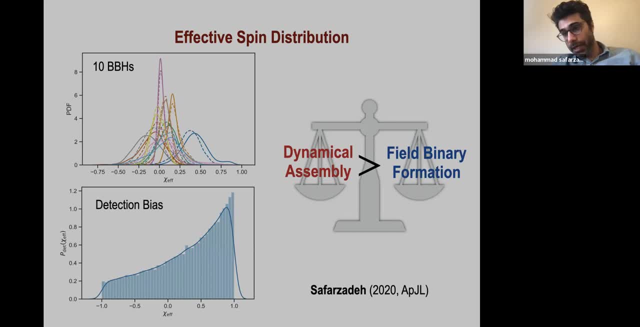 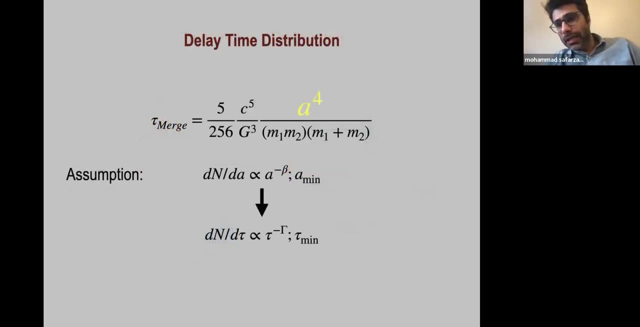 points to the fact that perhaps dynamical formation perhaps dominates the formation scenarios, But this is not the only way you can go after the formation channels. We know that. Sorry, could you go back to the last slide really quick? I just have a quick clarification question. 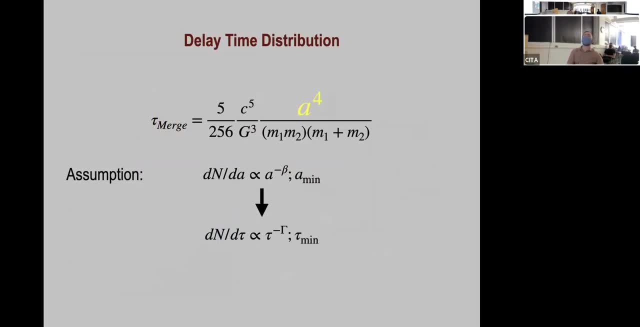 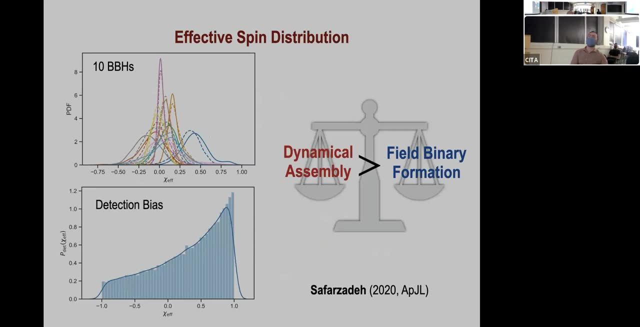 Yeah, So those constraints, So the constraints on the effective spin parameter, do those include the prior including the detection bias within them, Or do they not include the prior including the detection bias In order to infer anything from the chi-effective distributions? 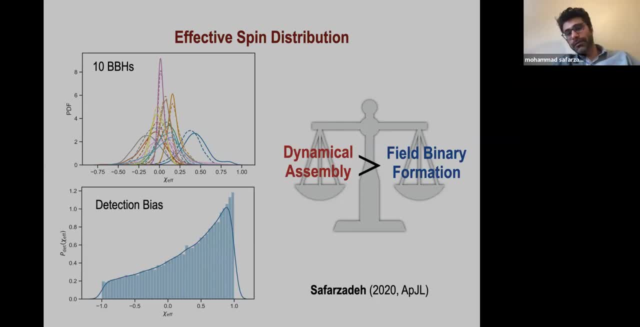 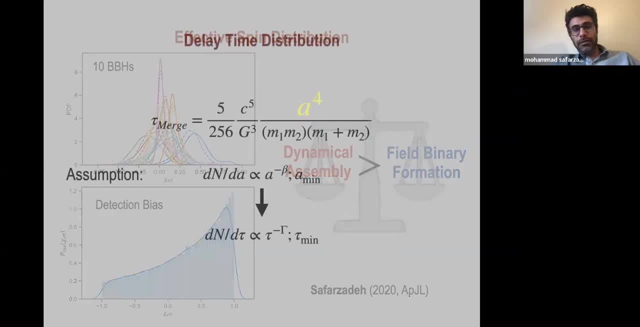 you have to take into account the detection bias If you remove the detection bias. yes, that's what I meant. Yeah, yeah, yeah, Sorry, Apologies, Thank you. There is a delay time distribution in another factor And that is a simple relation, that the time 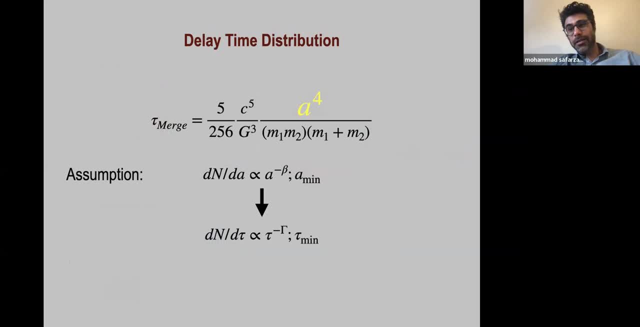 it takes for a binary to merge scales as their same major axis to the fourth power And if you assume that binaries are distributed logarithmically in separation, for example dn dA goes as a to the minus some power that will translate into the delay time dn dT to go. 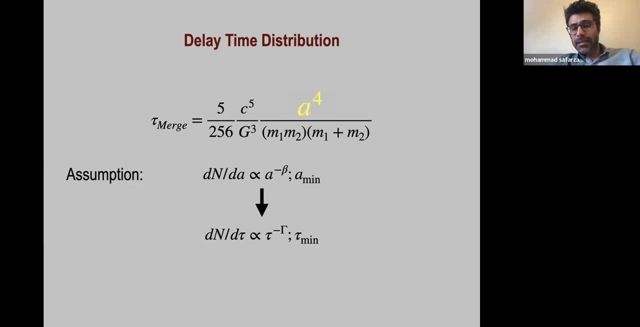 as t to the minus some power And these slopes, the power law slopes, or the minimum time for delay time, is related to the slope. you consider, for the separation and the minimum separation that you're asking for your population, The least complicated scenario to model the delay time. 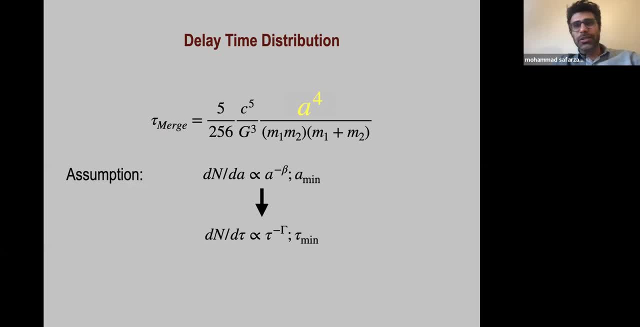 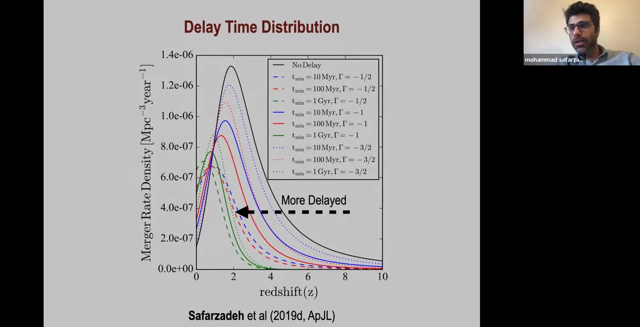 is basically these two parameters, tau, min and gamma, which is how steep is the distribution and what is the minimum delay time. For example, if you have the black line showing the formation distribution or formation rate as a function of redshift for your system. 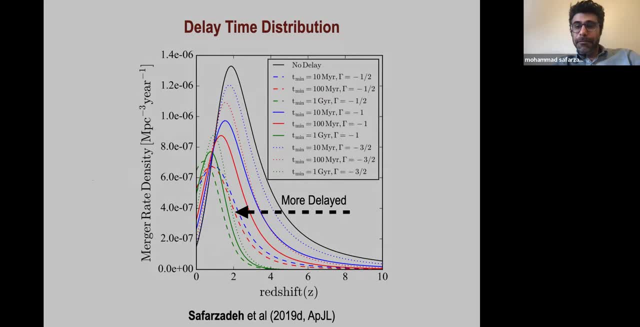 it can be any binary compact. object: different assumptions about delay, time, parameters, slope and the minimum time will predict different merger rate as a function of redshift. If you're more delayed you will get green lines. If you are less delayed, you will get the merger distribution. 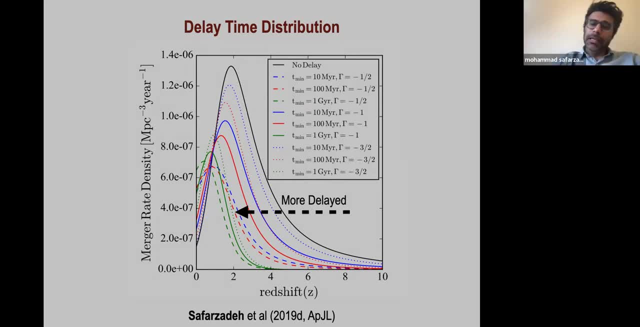 that is more close to the blue lines, et cetera. And then the question is: can you distinguish? I have just a quick question. So you have these two channels to make your tight binaries, And to me the dynamical channel will often. 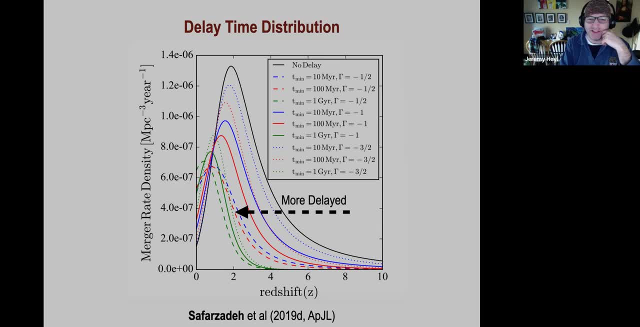 give you a binary with a large eccentricity, whereas the field one will give you a sort of circular binary. And your delay time doesn't mention the eccentricity at all. That's true. I said the simplest. Yes, that's true. 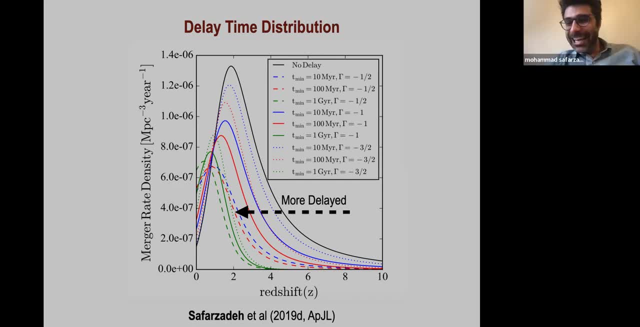 OK, It's like I've been doing this And then I will argue that even this is enough complicated To do it. But if you start with some Absolutely, I mean, it's really like the Perry center is super important, It's true. 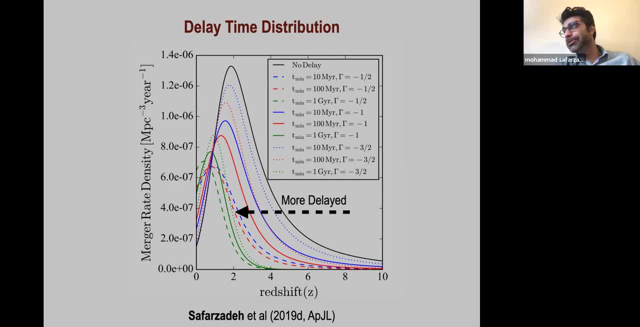 Yeah, Yeah, Yeah. The- including the eccentricity distribution will also be another factor And I don't know how it is going to affect it. It's going to push a little bit towards the show, So it's going to give a little bit of weight. 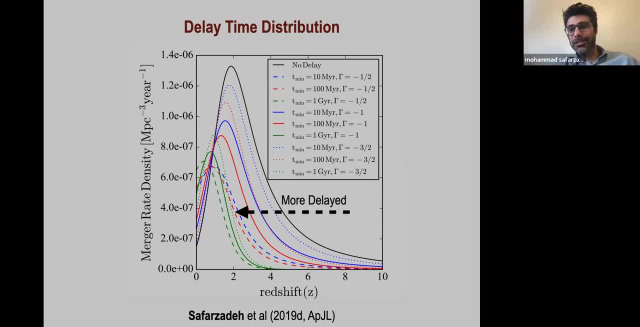 towards short delay times, But I don't know exactly how it's going to change the PDF of the merger time. Yeah, But I mean, I mean a simple calculation shows like you could start. You can make the delay time 100 times shorter or even more. 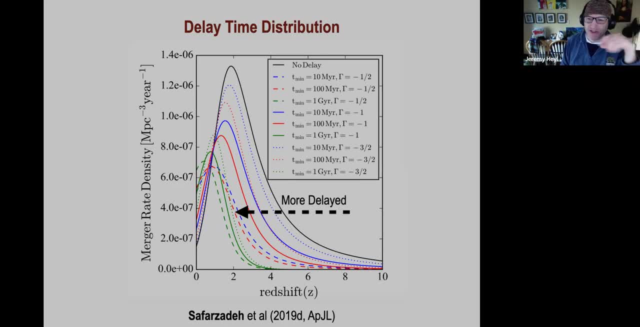 by starting with the same A, But You can make it a much, Or even a larger A, but have it be eccentric, Yes, Yes, It makes a dramatic difference. Absolutely, Absolutely correct. Yes. And also I mean then to the question: 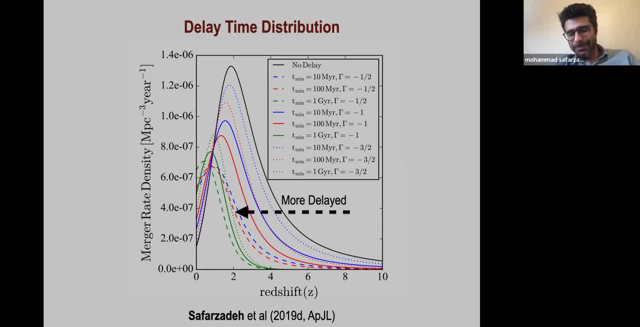 you can also get eccentric, of course, binaries in field formation scenarios through kicks, But then that becomes a very a topic that not everybody agrees about, Like people have Completely different opinions about the importance of kicks or whether it is related to only neutrinos. 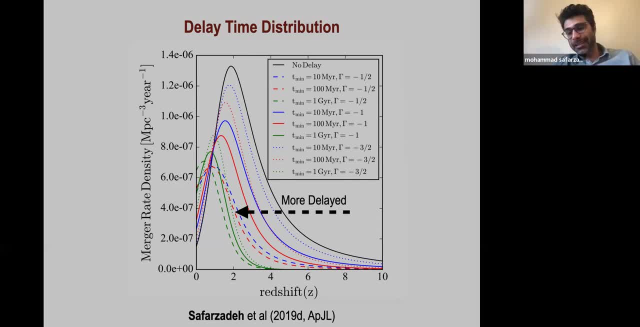 or only blackball, It becomes complicated. But I agree that the eccentricity will change the picture. But now I will discuss that this, even these two, constructing a delay time with two parameters is actually very. this one is even super hard to get at. 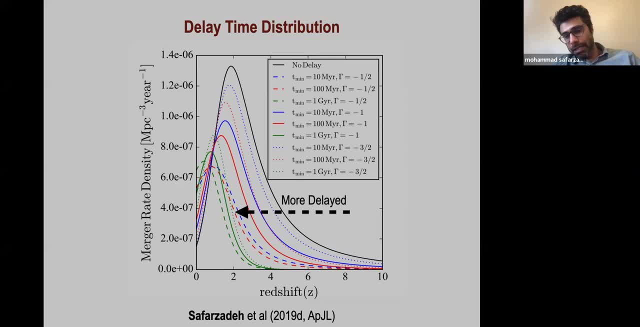 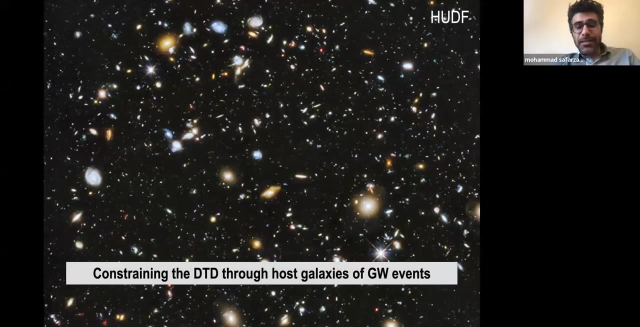 in the sense that I will describe next. So Let's imagine, this is the different plausible universes that you have And you want to tell apart, tell these curves apart, And one way to do this is by looking at the host galaxies of these events. 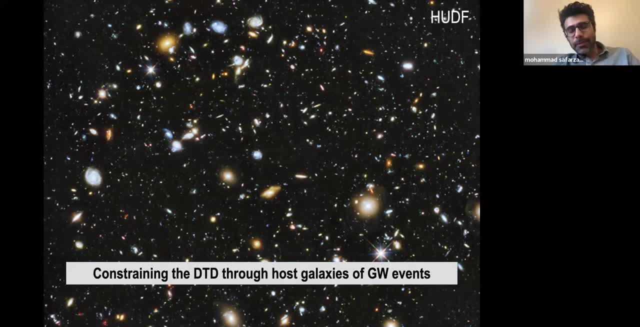 if these events produce electromagnetic counterparts, for example, like in a neutron star measure, right? So if you look at the host galaxies of these events- and we know from galaxy formation that some galaxies, some galaxies are red and some galaxies are blue- 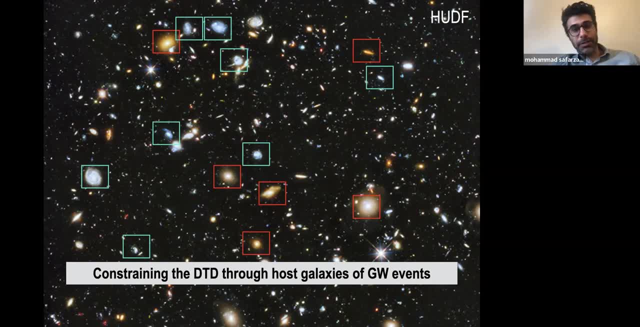 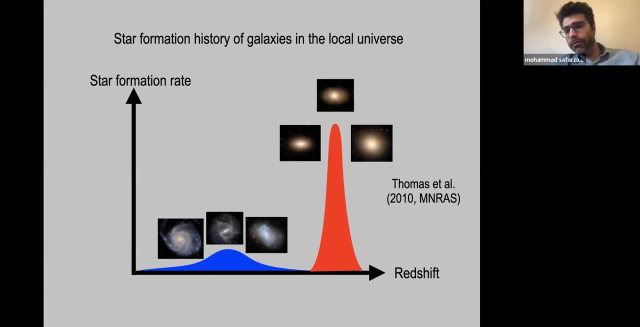 And these galaxies have had different star formation histories. We know that the red galaxies have formed at high redshift And since then they have used all of the gas supply they had for most of their stars And they have been dormant for a long time. 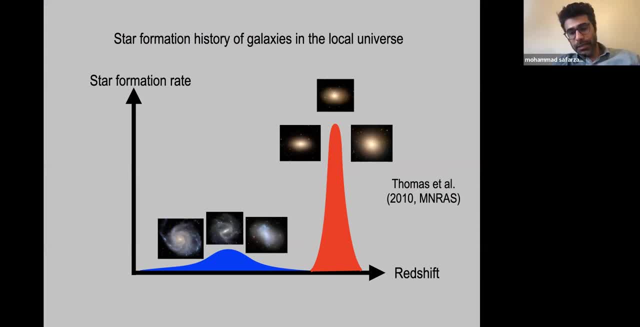 Unlike the blue galaxies that have more continuous star formation and they are younger systems on average, So So, So. So Now you have these formation channels. So, in order to predict the measured distribution of a class of binary compact objects, what you do? 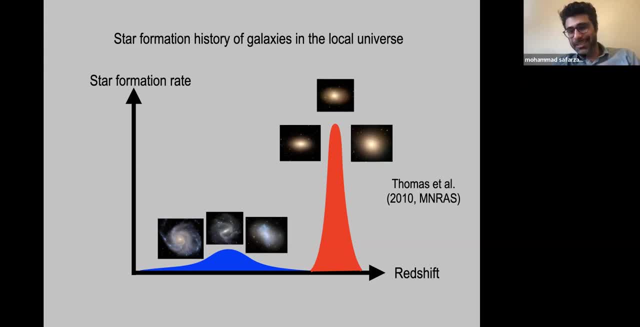 you convolve your formation redshift with a delayed time distribution And then you get the measured time distribution And you can see that convolving the blue and the red with a given delay time distribution will predict different distribution of measures as a function of redshift. 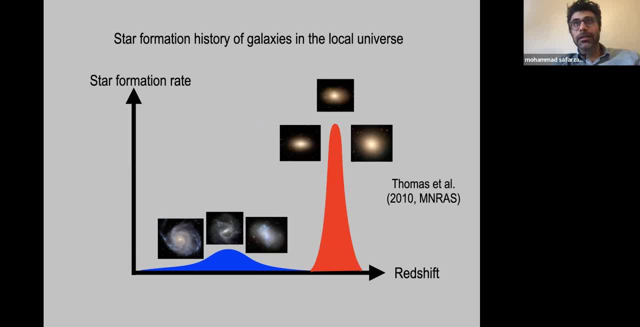 Maybe one example would be the following: Like imagine in the local universe, which is where all our observations are confined to. let's imagine that we see binary neutron stars only merging in red galaxies. Let's imagine we live in such a universe. 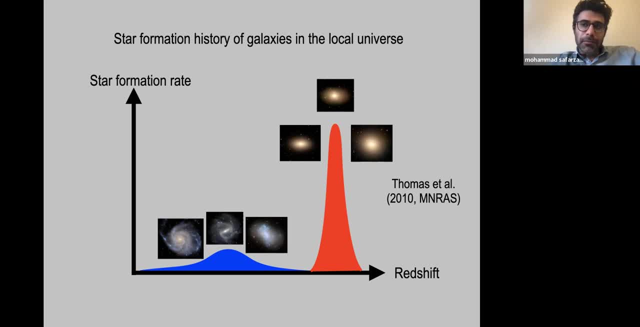 Now we know that they are dead systems. They haven't been a star from forming a star. They are stars for the past many giga years. If you only see all like most of your binary neutron stars merging red systems, that means that the delay time is long. 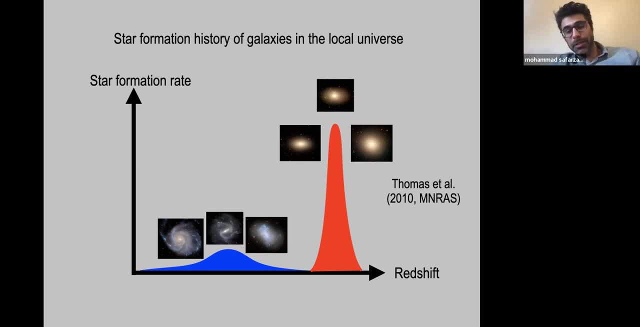 Because they are forming the scenario. the explanation would be that they are forming in all systems. They're also forming in blue systems, but it takes a long time for them to merge. That's why you don't see them in the local universe. 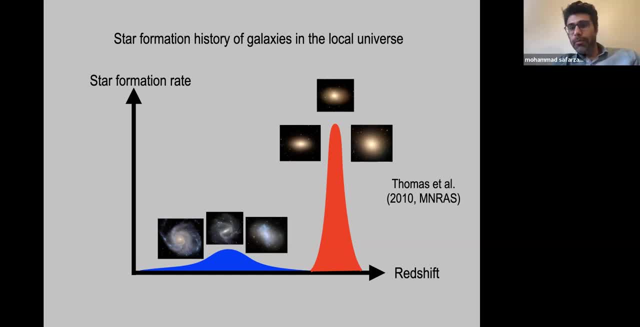 to happen for these systems to merge in blue systems. But since delay time is long and these red systems have formed in the early universe, now you can see them merging in such systems in the local universe. I hope this makes sense, but it's very simple. 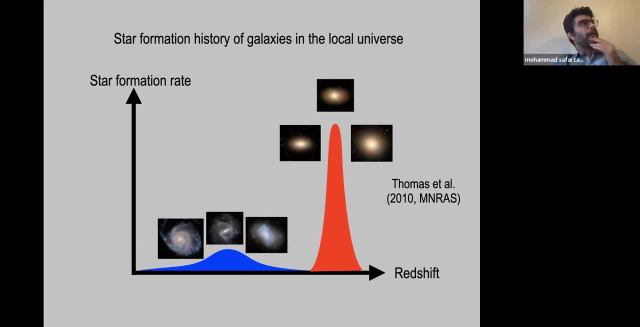 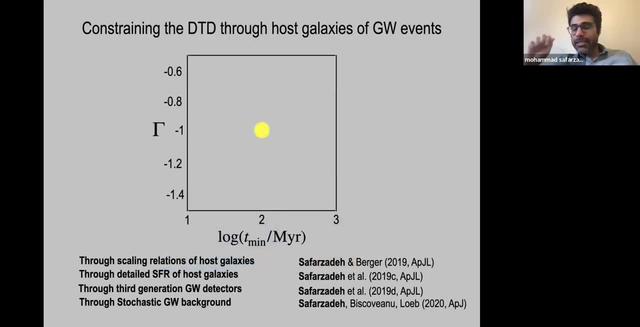 If I'm not clear, let me know and I'll explain further. Now let's imagine that we live in a universe with a particular delay time parameter. Let's imagine we have a t-min and a gamma, And let's imagine 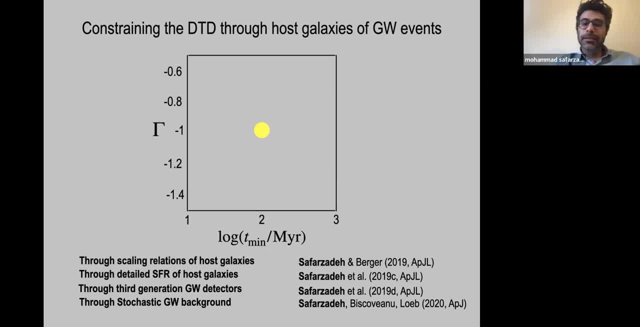 The universe is such that the yellow dot is the true parameter of your binary compact object. Now, by observing different number of host galaxies, like how these systems are merging different galaxies and what are their hosts, you can get closer and find this further like get closer to the yellow dot. 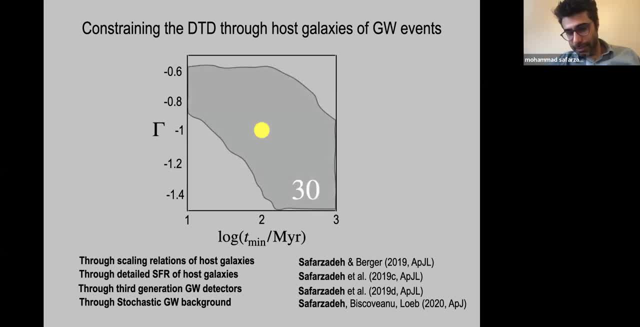 For example, if you only observe 30 systems, this is the confinement, This is the posterior distribution you get for t-min and gamma. If you observe 100 systems, you get the tighter constraint And you get 300 systems, then you 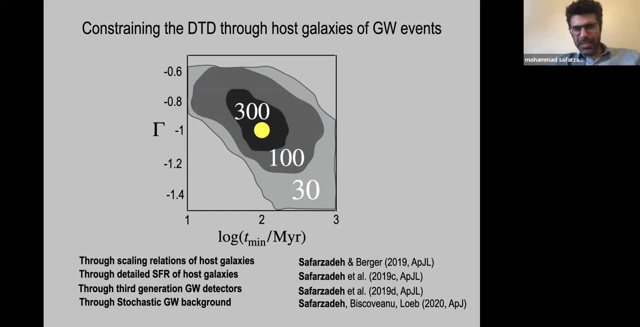 get a really tight constraint to within 10%, 10% or 20%. So you kind of need hundreds of these binary neutron stars with electromagnetic counterparts to be detected in the local universe so that you can go, after the delay time, distribution parameters in its simplest form, to the accuracy of 20%. 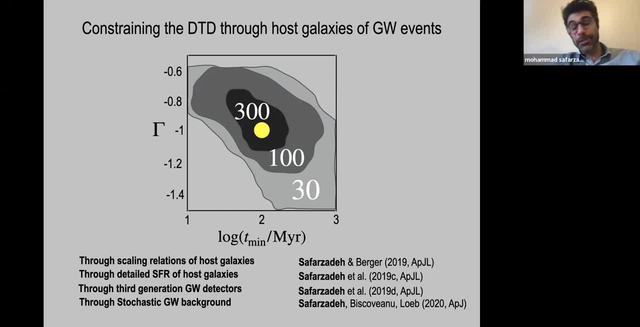 And currently we only have one detected system with its host known right: 17 over 817.. And this kind of shows you how hard and difficult this is to actually go after delay time distribution, which says actually everything about how these systems may. 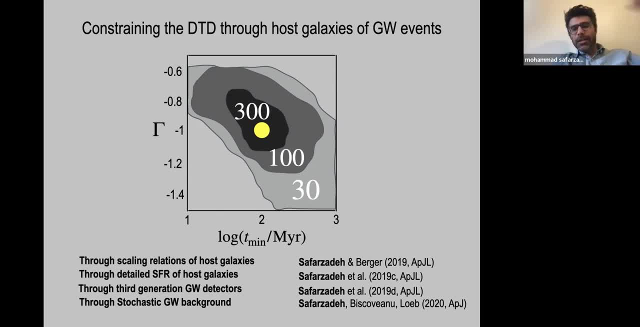 merge over across redshift. There are different ways that I have discussed in various different papers about OK, how can we go after this, through observing a stochastic gravitational wave background, or different approaches to the host galaxies, But all of them point to the fact. 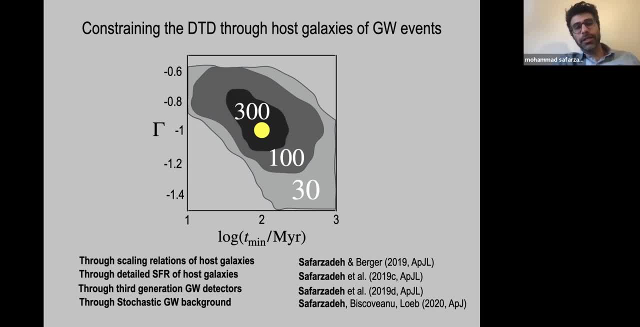 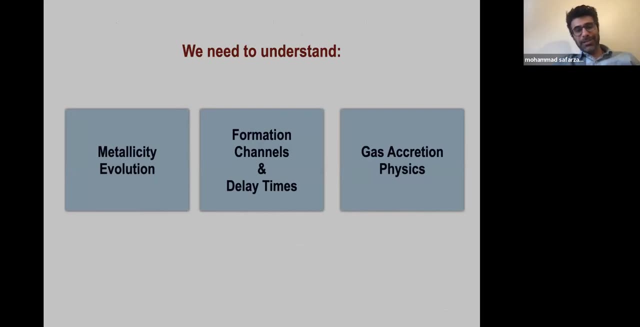 that we are not yet there to actually constrain in the simplest form the parameters of the delay time distribution. So that's it. That's enough for this, And then let's go to the next chapter of this talk, which is basically. I want to talk about metallicity evolution. 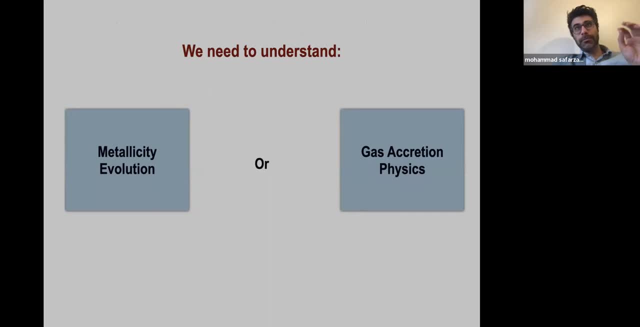 or gas accretion physics, Because I told you guys that the mass scale of a black hole depends on this progenitor's metallicity, So that we know. But also you can make very massive black holes by gas accretion. That also we know. 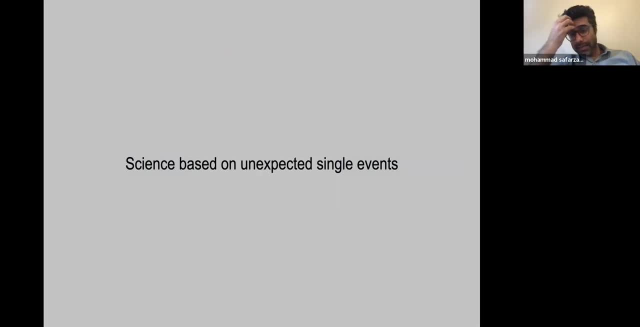 So now the question is: what is this? What is this? What is happening in the universe? If you see a massive system, how can we tell apart if it is formed from a low metallicity progenitor or is it formed from a high metallicity progenitor? 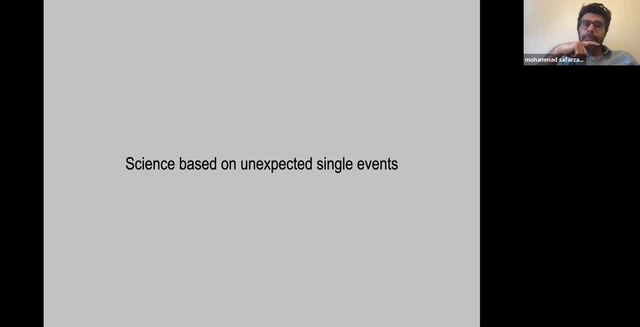 but has been accreting gas. OK, so let's go to the single event that has been observed. The most massive binary black hole that I will talk about is a system that was found in the first observation after the first black hole. 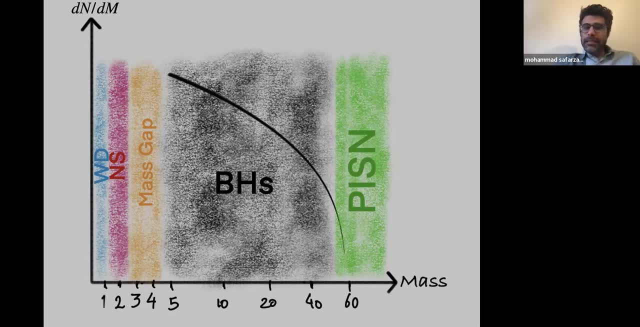 The first half of the third observing run. But I will start this by showing what was expected for black holes, what was expected for the mass function of black holes. So if you plot the mass of black holes or the mass function of black holes, 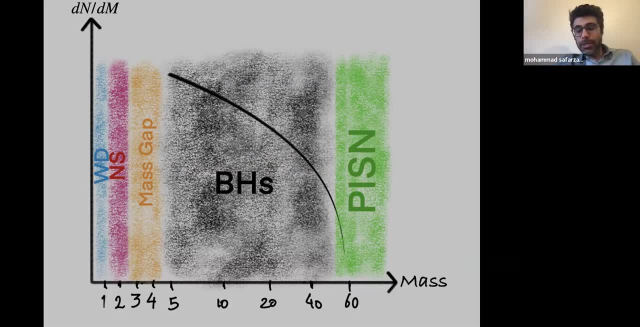 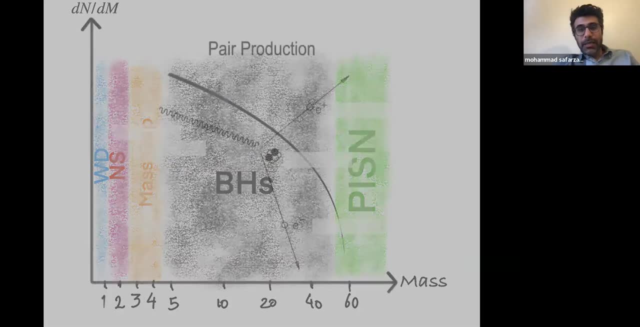 there was an expectation that the black hole mass spectrum is going to cut around 40, 50 solar mass and due to a process called peri-instability supernovae, And the process is that you have a photon And this photon will create pairs. 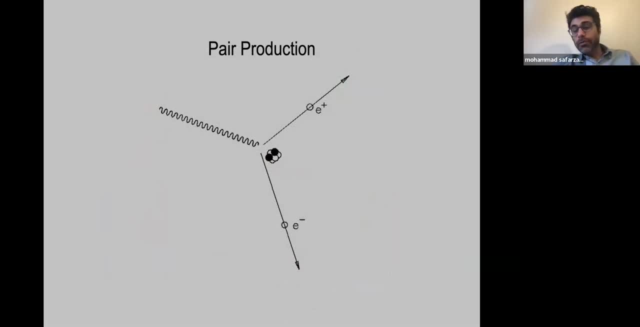 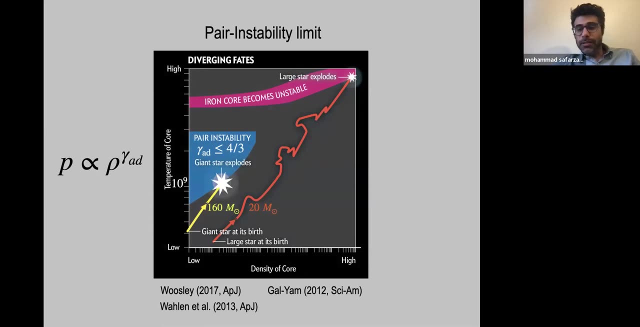 of electrons and positrons in the presence of a nuclei And this is detrimental to the future of a star because, for example, if you're 160 solar mass, shown with the yellow line, and if you plot this evolution of such a star, 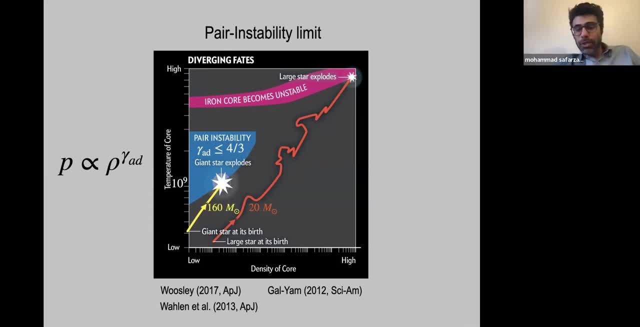 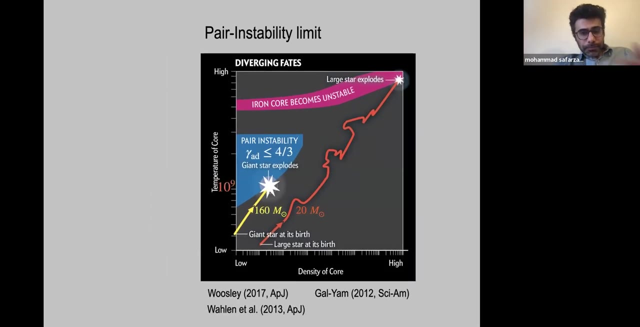 in density, temperature of the core. the star evolves, But it will hit an island of instability where the adiabatic index falls below 4,000.. And so what is happening are two things. One is that we have to note that the temperature at which this 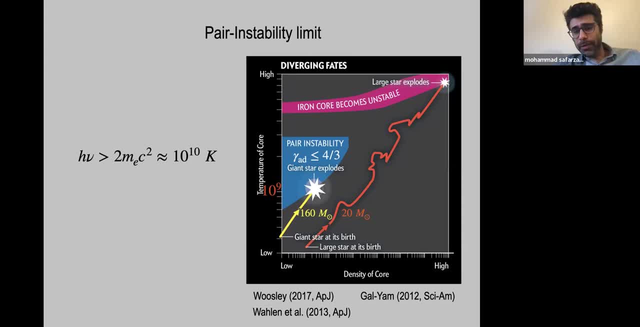 happens is about 10 to the 9.. But in order to produce a pair of positron and electron, you need about 10 to the 10K Kelvin. And now the reason this still happens at 10 to the 9 Kelvin is that all these photons belong to the tail of the point. 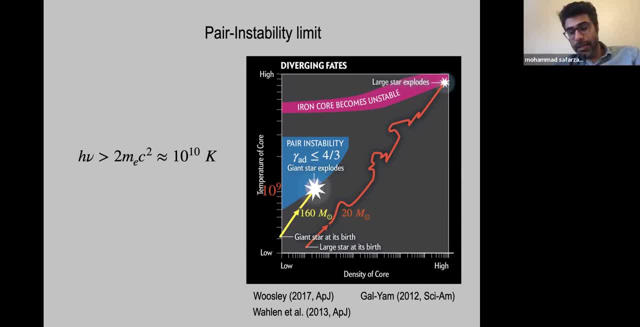 distribution. So that is why you still get it at 10 to the 9.. And what happens is that you have a pair of production. These pairs are not relativistic. They are basically like deadweights And they basically remove the radiation support. 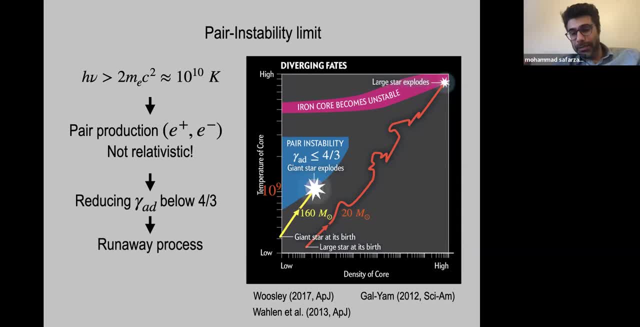 from the core of the star. The star shrinks. due to the heavy weight of the star, The core shrinks. This shrinkage leads to boost the temperature higher. But this is again not. It's not going to work, because then you 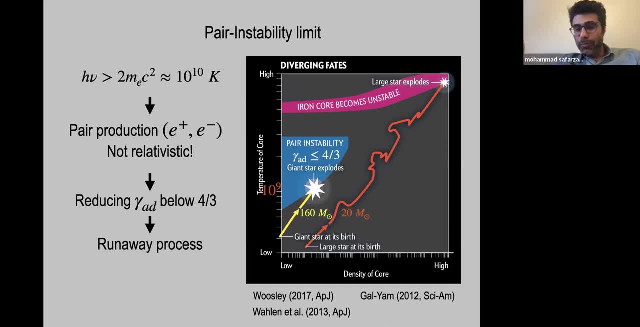 produce even more pairs. So again you produce more pairs, You reduce the pressure support, And this is a bad cycle which leads to a runaway process at the end of which the whole star explodes. So this pair instability issue will result in black holes, of having basically black holes. 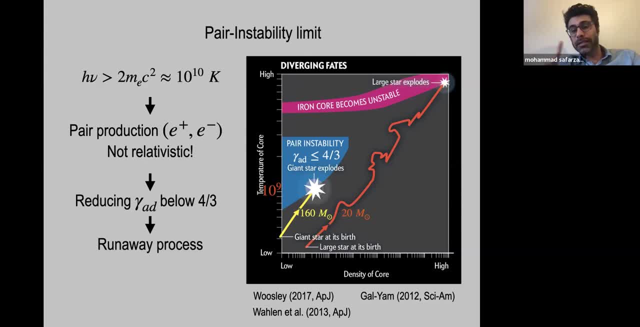 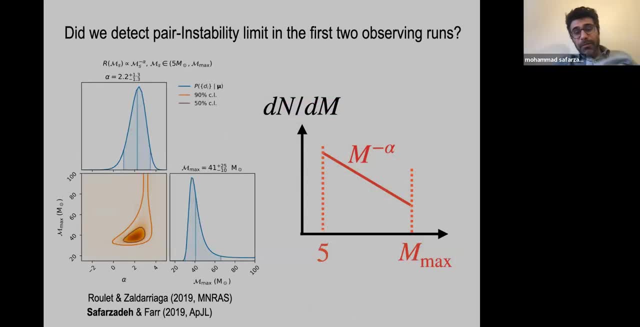 with maximum mass around 45 solar mass. We're born from a single star And people were very happy by analyzing the first 10 black holes of LIGO discovered in the first observing round, And what was discovered was that, oh, there is about a maximum mass above 41 solar mass. 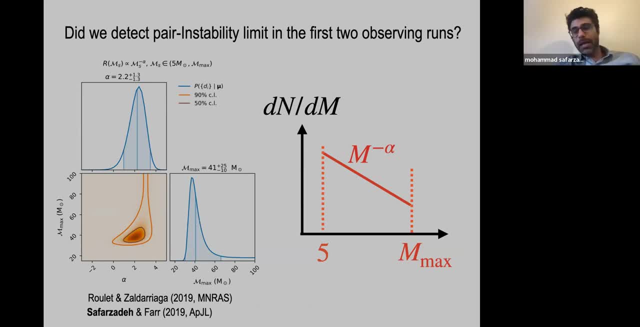 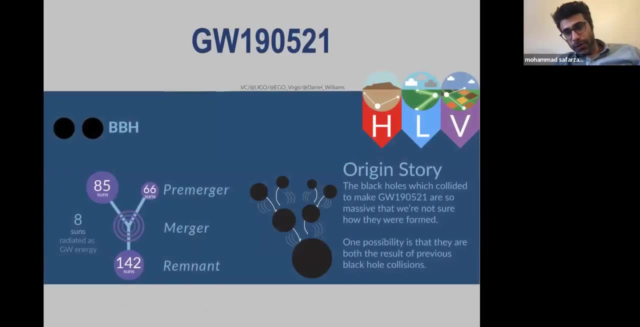 Stan Woosley and collaborators are correct: There is a maximum mass. But soon after this was challenged by the discovery of LIGO, It was a failure. discovery of 190521, which is a 85 solar mass and a 66 solar mass, So both of them are outside. 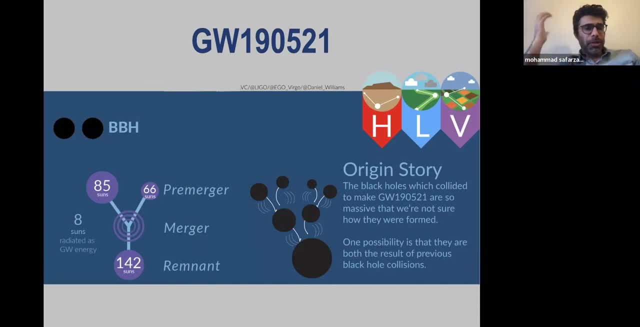 the pair instability limit, People originally argued that both of them are assembled dynamically. but there are many issues with assembling dynamically each one of these black holes, because when you do assemble black holes this way, the resulting black hole will receive a kick and it is hard to confine both black holes in a system and then again bring them. 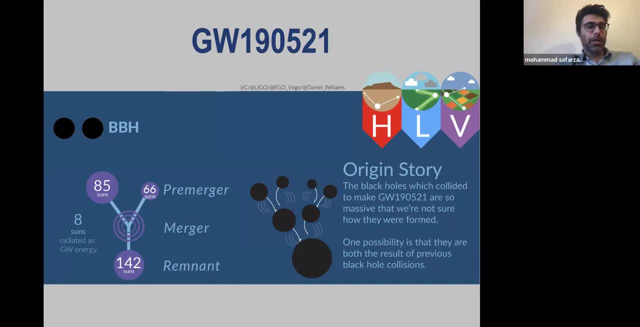 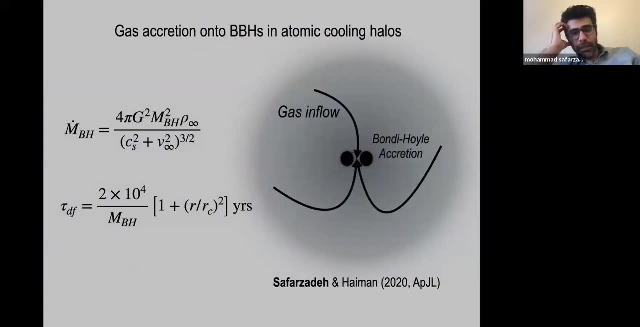 together to make more massive black holes. So this is a very fine-tuned scenario if it had been forming dynamically. What we suggested with Zoltan Hyman is that we have a binary system and both black holes are about 40, 50 solar mass when they are born. but there 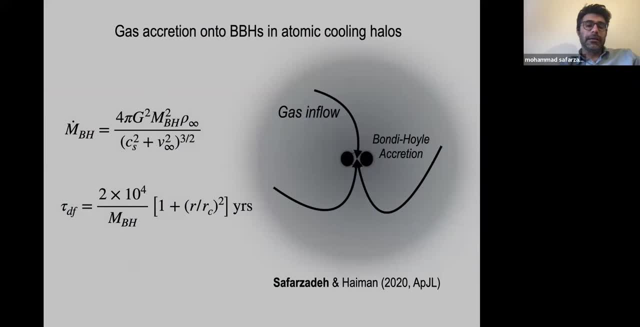 is a gas inflow where they reside and they accrete. This can easily happen in the core of atomic cooling halos at high Redshift, which are very, very dense systems. What we showed with Zoltan Hyman is that if you have a binary 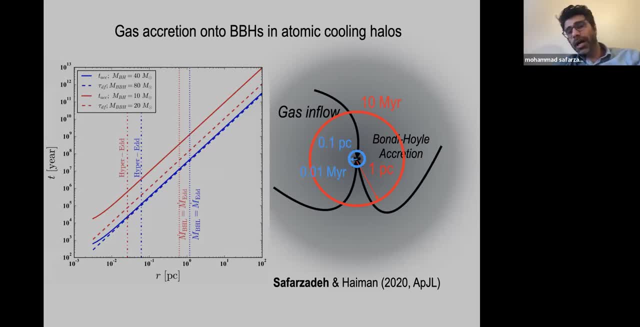 black hole and if they reside, for example, within 0.1 per sec of an atomic cooling halo, you can actually double their mass in a matter of 0.1. percent of a million year, or if you are within a parsec. 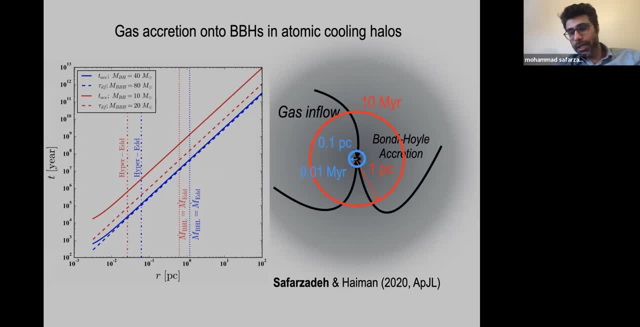 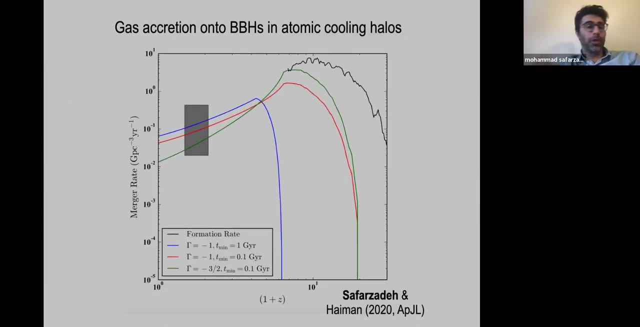 of at the core of atomic cooling halo. within 10 million year you can actually accrete enough to double their mass. So this is helpful And we said that, look, we don't know the delay time for this system, but we played around different plausible delay times. 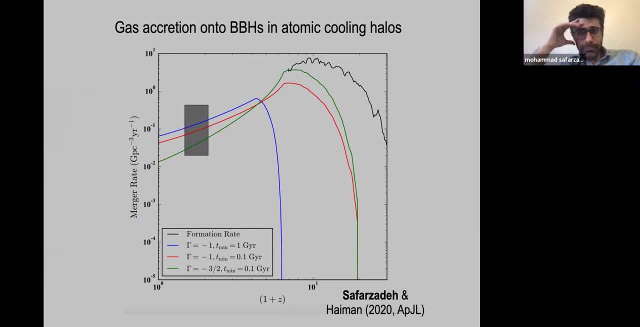 and all of them showed that, if you assume these systems are born from population, three of stars that are shown with black line, the merger times of which are shown with colored lines, all predict a rate that is consistent with the observed rate of such systems. And we said: okay, so this is still a plausible scenario. 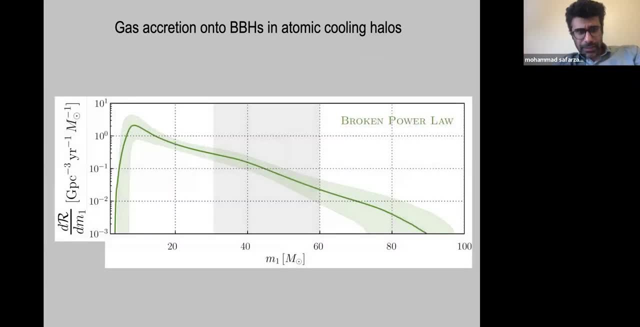 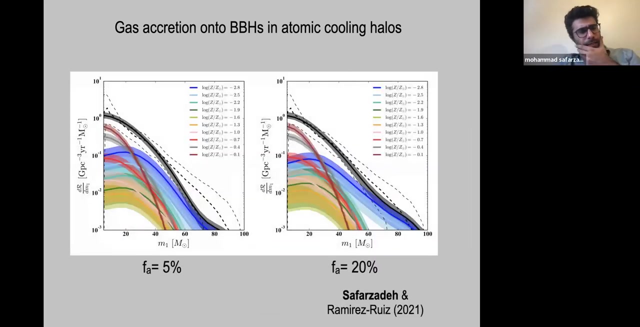 And later on, in 03,, the black hole. due to discoveries of such systems, the blast hole max mass function was revised and now it easily extends to 100 solar mass. and the question is: can we explain the observed black hole mass function? and a work that i did with enrico ramirez ruiz- is that we assumed 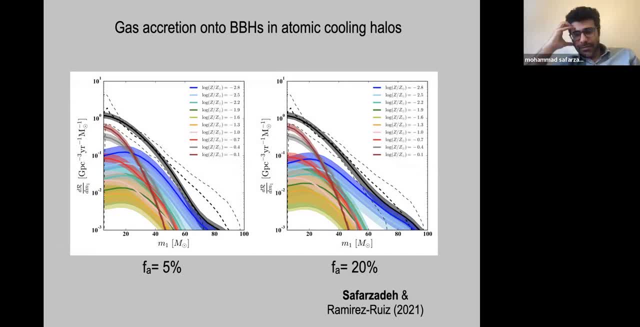 five percent or two, twenty percent of black holes that are formed in the early universe to double their mass, uh through gas activation and uh, and what we show here is that the black line, with its uh, with shaded region, matches the dot that the regions of the dotted region is the 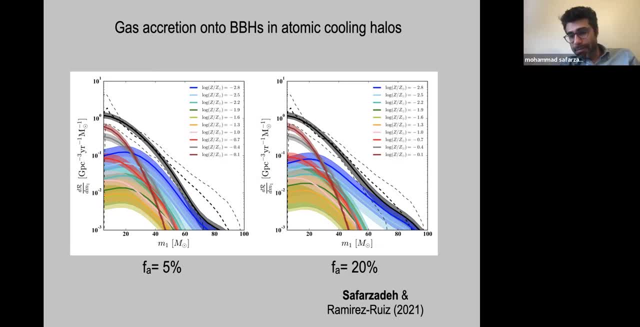 is the plus the mass function, the observed mass function and the colored ones are the ones show our model. So what we show is that the black line in our model is consistent with the observed black hole mass function if at least 5% of the black holes 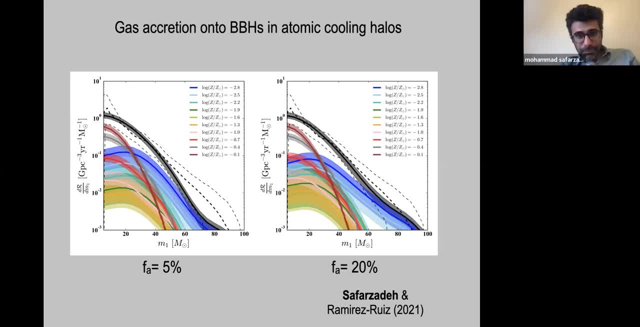 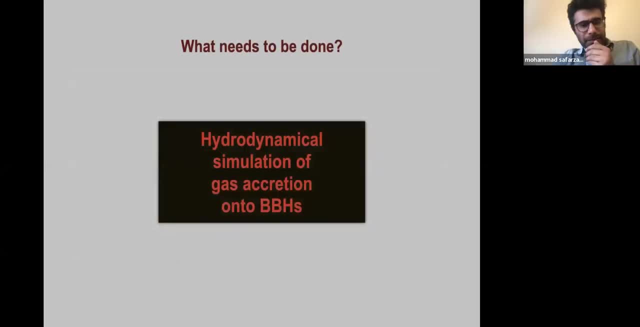 of the formaldehyde redshift double their mass through gas secretion, which was interesting. So, however, there are issues with this scenario of gas secretions into binary black holes that require further simulations of gas secretion into binary black holes that we are working on. 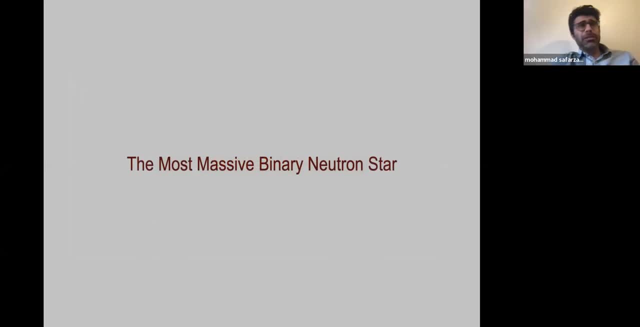 But the issue is not just the massive binary black holes. There's also the most massive binary neutrinos that I referred to in the beginning of the talk, And that is 1904-25, with a total mass of 3.4 solar pounds. 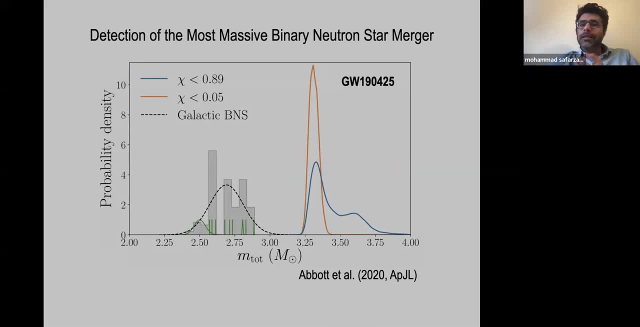 Now, This is a different, Different system. We are not sure if this can be formed through gas secretion, But let's talk about some plausible scenarios. So when this system was formed, everybody was shocked And people had different ideas. And one of the ideas of the LIGO's paper out. 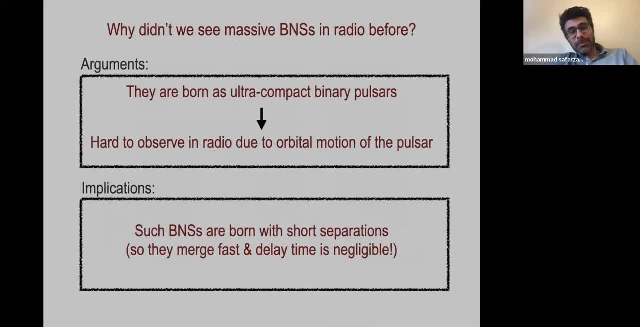 was that this system has been born as an ultra-compact binary pulsar, And this is why it has been previously missed in radio observation, Because this, due to being in a compact binary with very short separation, the detection of the pulses of the pulsar is smeared out. 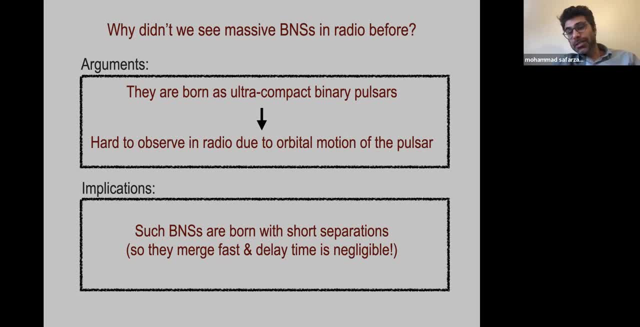 And this is very hard for the observers to detect such systems. The implication of this is that such binary neutron stars are born, of course, with short separation, But the implication is they merge fast, So the delay time is very short. So the delay time is very short. 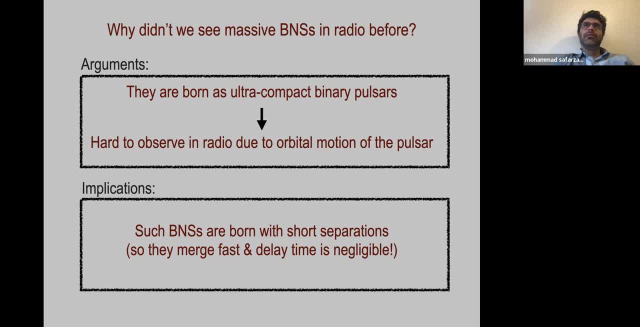 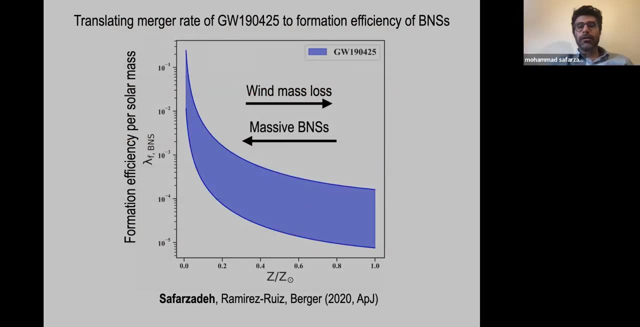 Now, OK, so why can this not be a good explanation of the system? The reason that this is perhaps wrong argument is the following: We know that, due to the wind mass loss that changes with metallicity, more massive neutron stars can form from less metal-enriched stars- progenitor stars. 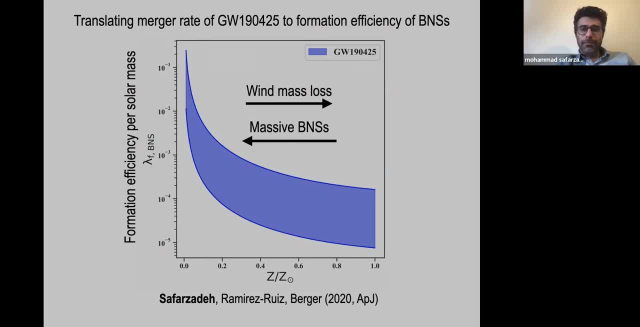 So if you want to make a massive binary neutron star, you better be forming them from a low mass progenitor. But this system has been observed locally And that line of argument is saying that the delay time is short. If the delay time is short for these systems, 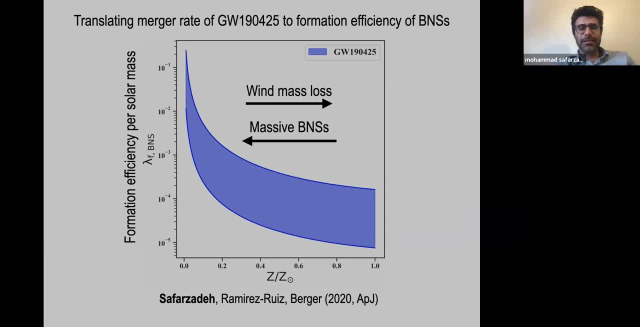 and we know in the local universe that the metallicity is high. the chances that this system has been formed from a high metallicity progenitor is actually very high. But we know from a high metallicity progenitor we don't get massive binary neutron stars. 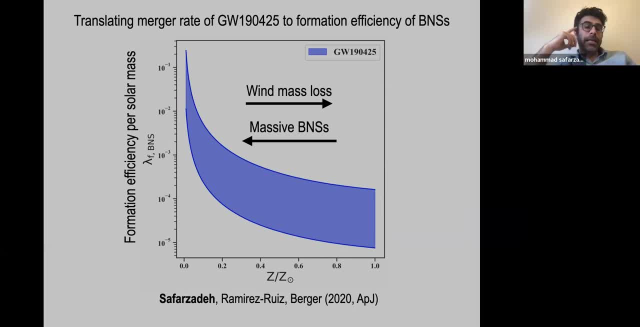 So that is a conflict. And if you want to make such systems from low metallicity progenitors and if you basically invert how much the star formation in the local universe is taking place at low metallicities, you will get very high efficiency For such systems to form, because the star formation at low metallicities is very rare. Now you want such systems to form from low metallicities, And that would imply the very high formation efficiency of around 10 to the minus 3 solar mass, 10 to the minus 3 per solar mass. 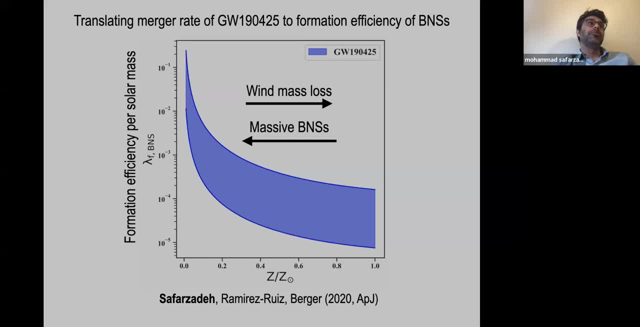 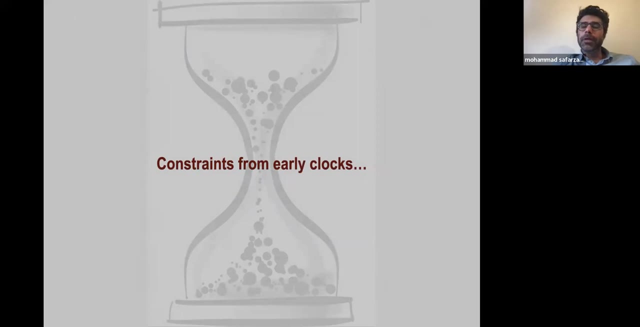 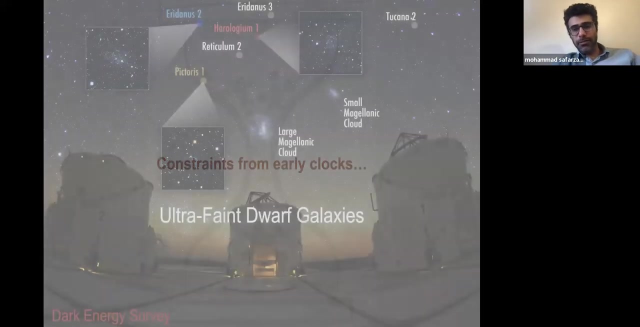 Now I will argue In the next slide that this is insane, this such formation efficiencies, And the reason is that we have some constraints for formation efficiencies of binary neutron stars from ultra-fine dwarf galaxies. So what are they? So ultra-fine dwarf galaxies are satellites of the Milky Way. 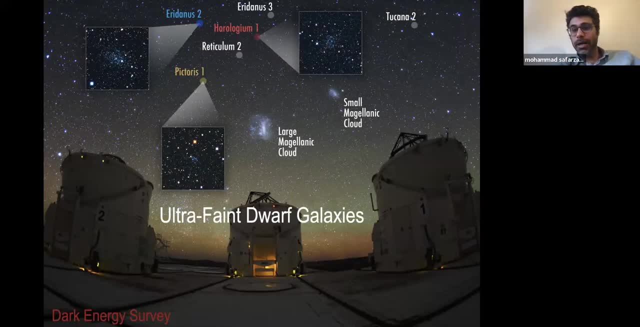 that are believed to have formed very early on and sees their star formation. Some are dead since Redshift 6 or 7.. And these are routinely being found in dark energy survey And in one of them, namely reticulum 2,. 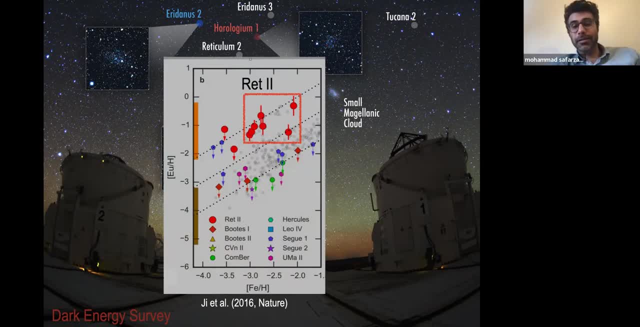 we see like seven of their stars have been observed to be polluted with europium, which is an element that is generated when two neutron stars merge. At least this is the leading theory, Which means that in reticulum 2, which is a system that is dead since, let's say, Redshift 6,, 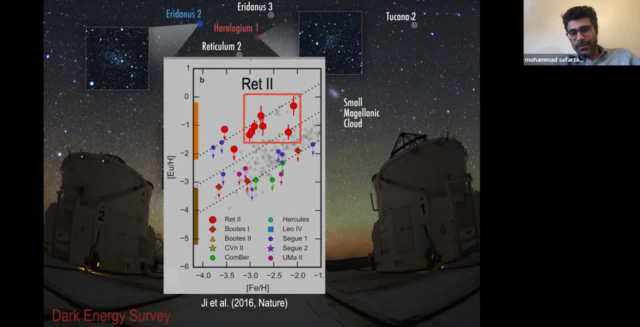 in that one giga year time life that it had by then, there has been a neutron star binary formed, merged, polluted the medium with europium, Newer stars formed from this gas. Now we see them in their spectra. So this gives you a constraint and formation efficiency. 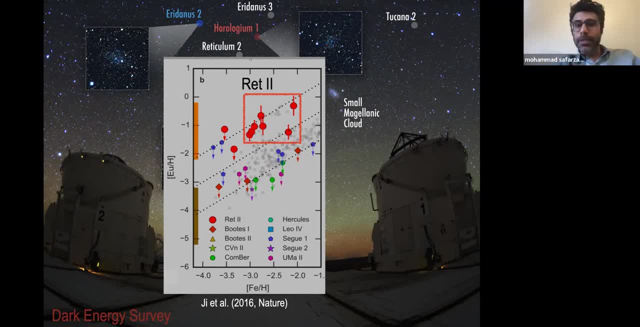 of binary neutron stars at low metallicities, because these systems again are very high rate of systems And we know that the metallicity back then has been extremely low. And also we know that the metallicity of these stars, we know it's like hundreds. 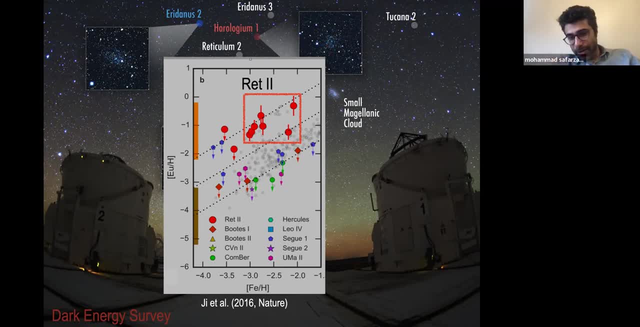 So the x-axis is hundreds, So it's like a hundred, And the y-axis is showing the metallicity And the y-axis is showing the europium. So we know that these are very metal-poor systems, but it's still enriching europium. 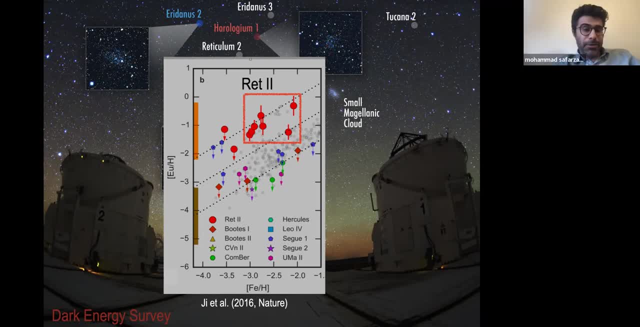 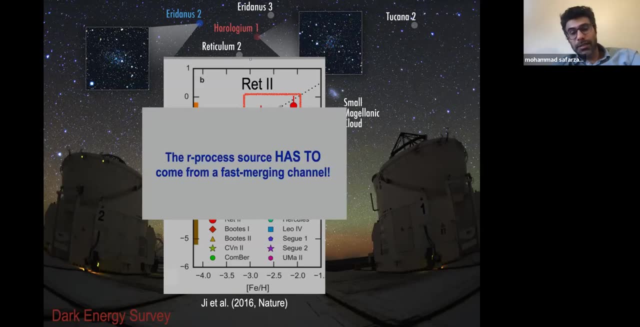 So this gives you the formation efficiency of binary neutron stars at low metallicities, with the implication that this has to be a fast-merging channel. Whatever led to the formation of our process elements, we know that it's going to be very, very fast-moving in this galaxy. 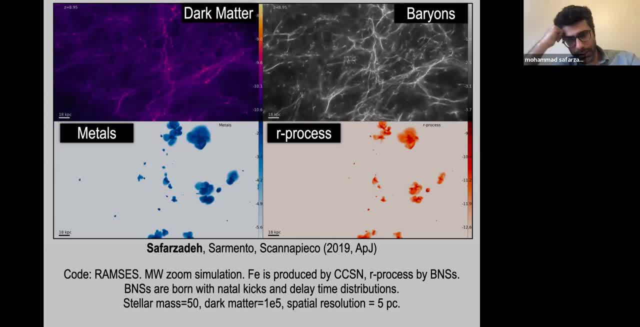 So we did in 2018, I did some zoom hydrodynamical simulation. I don't show the movies because the movie, when I show it, the whole thing freezes, So I just took a snapshot of it. It's just dark matter, baryons and metals, and also our process. 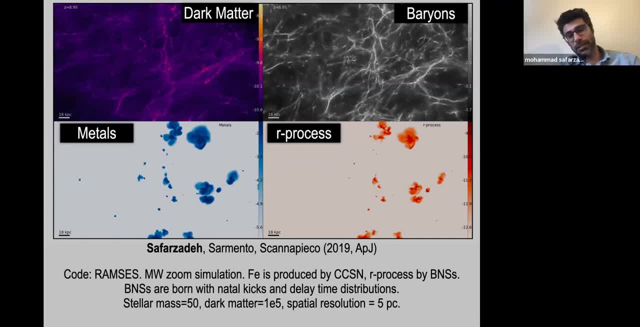 which is generated by the binary neutron stars that we simulated. in the simulation It's a stochastic star formation scenario And then, with some formation efficiencies, we tagged some of the stars as binary neutron stars, which will receive a kick with the delay time. 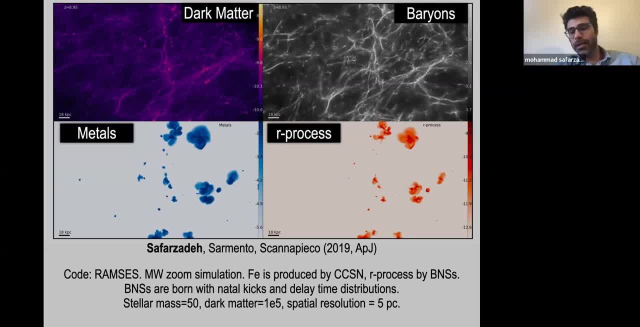 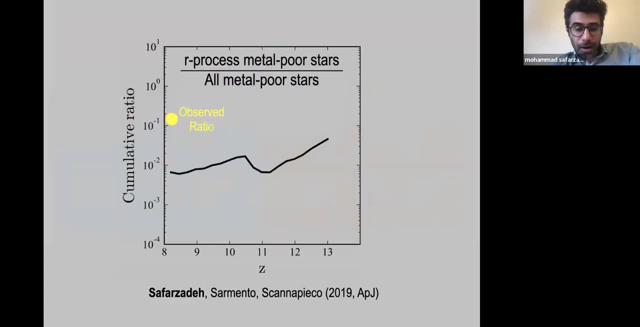 And then when they merge instead of metals, they're going to pollute the medium with our process. So we do these simulations And then we look at the distribution of the stars in our process And what we saw is that the observed ratio 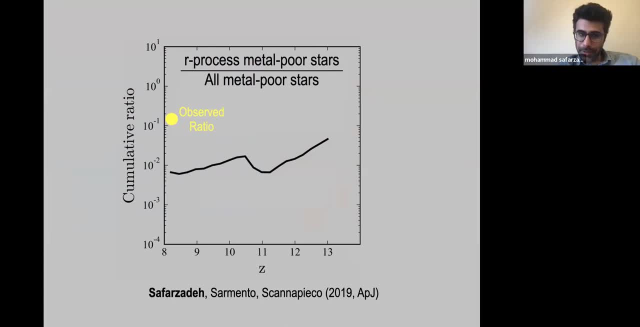 of our process metal pore stars to all metal pore stars- is much higher than what we got from our simulation. And what we got from our simulation was assuming the most optimum yield for our process materials And the only way for us to do that. I'm not sure, but we did it. 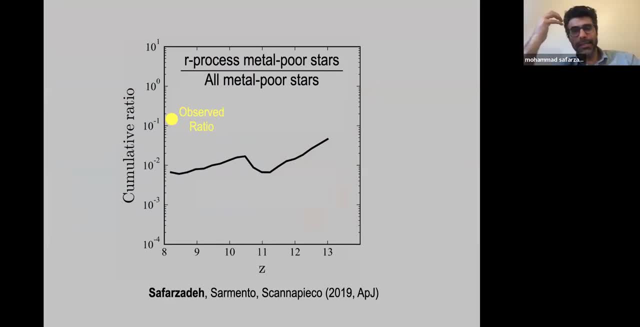 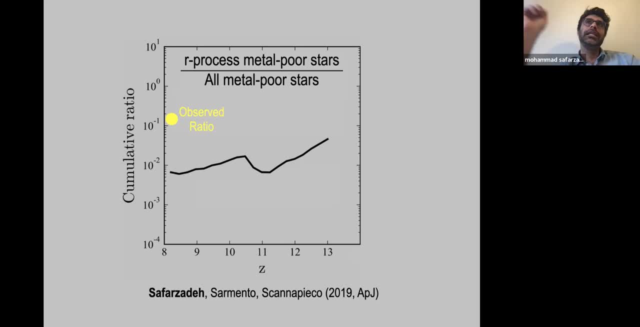 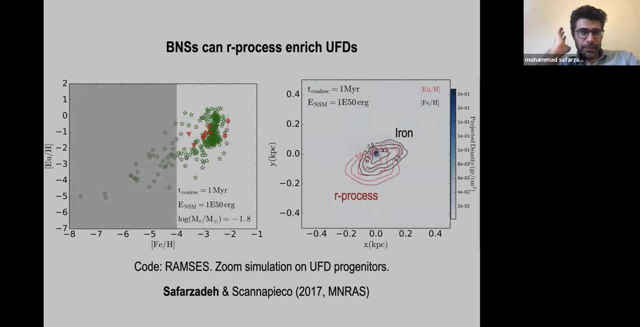 that are formed in nature at low metallicities, basically meaning that we need it to inject fast merging channel binary neutron stars by hand into the simulation so that we match the observed ratio. these simulations. the issue, and one other issue that we need to be careful about, is that binary 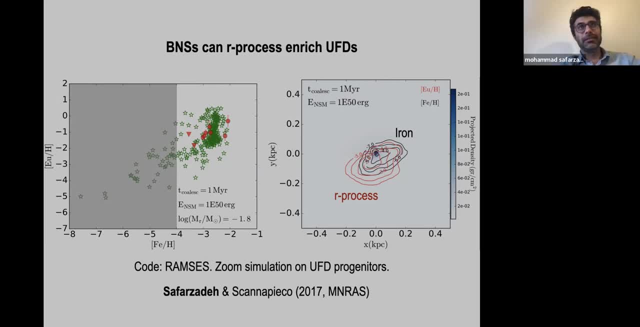 neutron stars are born with kick velocities, so if there is no kick, this was the distribution that we found in one of our dwarf galaxies. that, for example, this is how our process material and iron are distributed in the gas, and on the left panel, how the stars are distributed in europium. 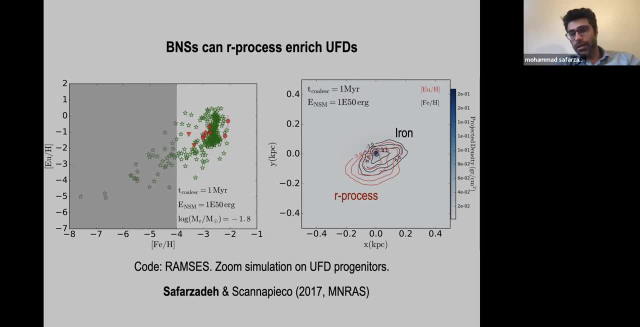 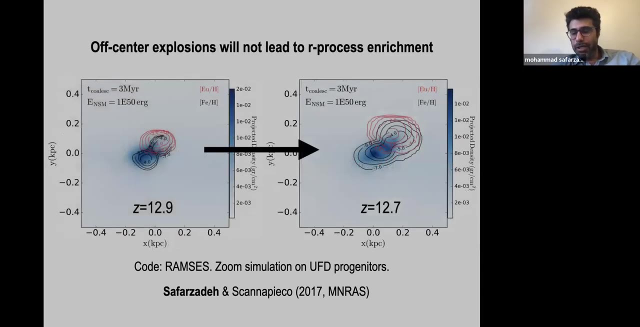 versus iron distribution and over plotted are the stars of reticulum 2.. so the green are the stars from simulation, and then the and then the red are the stars that are observed in reticulum 2, but if, if, if the explosion happens off center, which had in one of our, in one of the systems, 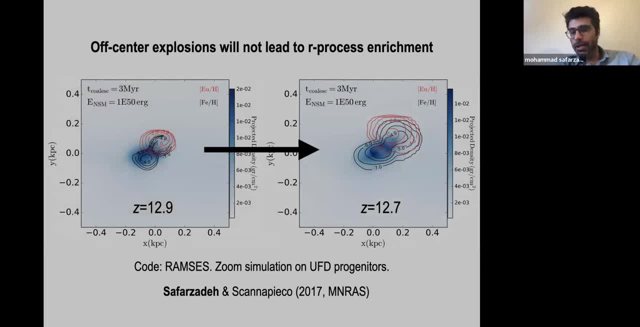 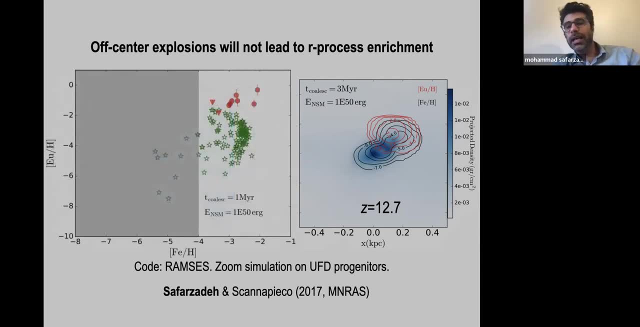 this is what happens, so that the distribution of european and iron are not, uh, co-centric, then what you get for your stars is that they are not really enriched in our process as much as they could be if there was no kick, which is obvious because now your, the our process material is too diluted before the next generation can next generation. 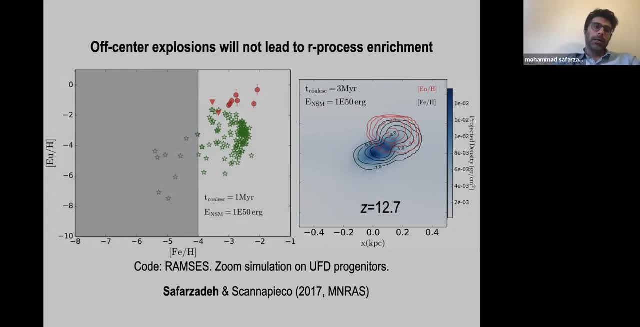 of stars are born and inherently european. um, so that is why, uh, we needed the fast emerging channels. uh, because, although you're gonna form and and uh and eject our process material, but you're gonna produce this, our process material irrelevant, like outside the galaxy, which is not going to contribute to our process enrichment of the system. so, um, 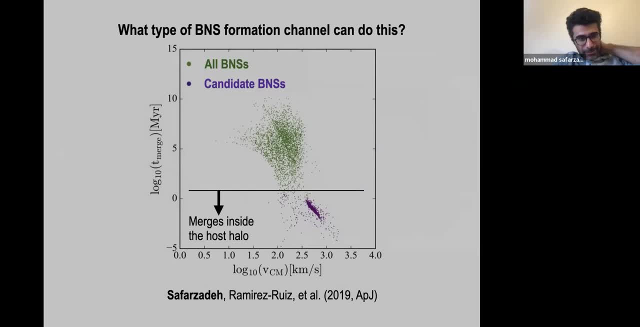 this uh leads to some discussion about, okay, what section or what part of the parameters? but in terms of delay, time and kick velocity, can the binary neutron stars have in order to enrich a small system or reticulum too? and one can see that those that can enrich basically do have very high kick velocities. but 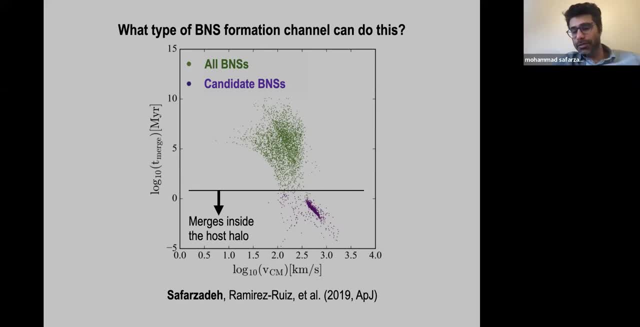 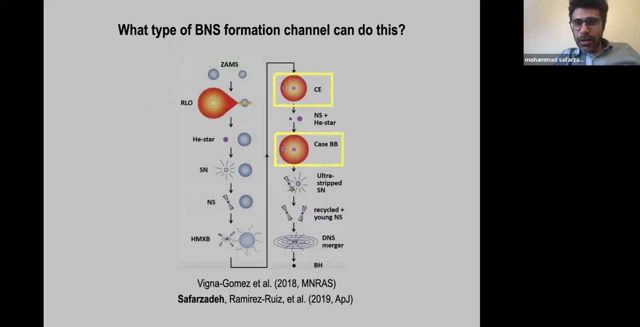 have very, extremely short, short managing time. those are the ones that merge inside the halo that can lead to our process, enrichment and and there are scenarios that can lead to such systems, but they are not mainstream. they're not. so there is this case pb mass trans, this case pb um- binary formation scenario, but these are not. 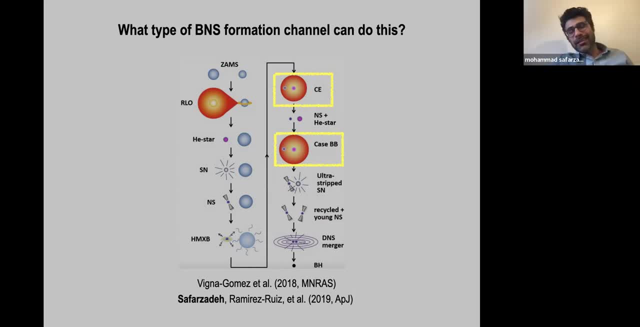 these are not mainstream ideas, and some people uh argue whether this is physical or whether this is not physical, but regardless, what we get is that we do need processes that generate extremely short period binaries, uh at low metallicities, in order to explain a satellite like reticulum too. 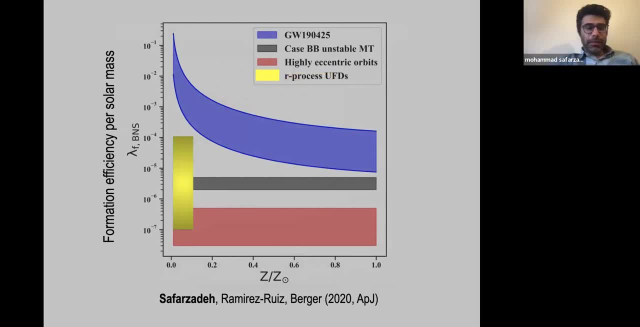 um, putting all of this together, what we, what we get, is the following: our process, ultra fenders, galaxies. they have a range for what is the efficiency of formation of binary neutrinos as low metallicities, which is shown in yellow? The blue is the constraints that you 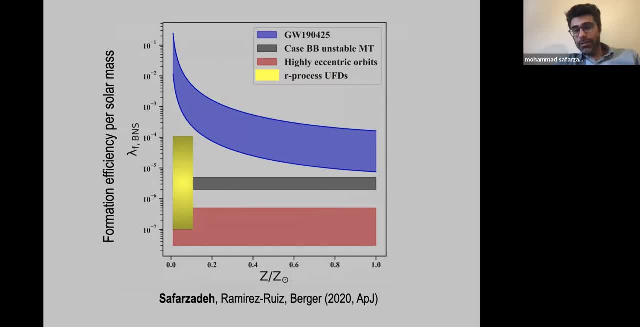 get from the gravitational wave detection of the binary neutron star, And the other lines are basically showing different, non-mainstream formation of short binary neutron stars. So what we get at the end is that it doesn't match. You cannot actually get to such extremely high formation. 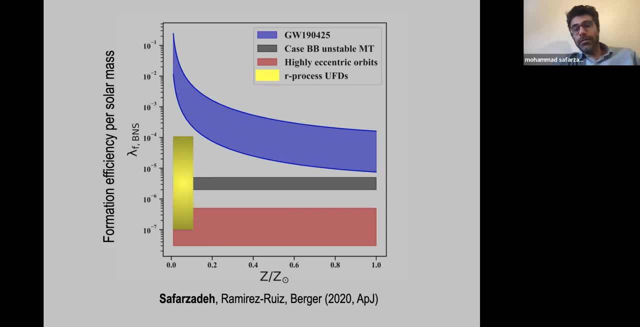 efficiencies as is implied by this gravitational wave detection, specifically at low metallicities. So that challenges that interpretation. Now, yeah, OK. and then I always argue that this can be itself a good topic for a PhD- is to do actual cosmological hydrosimulation in a survey. 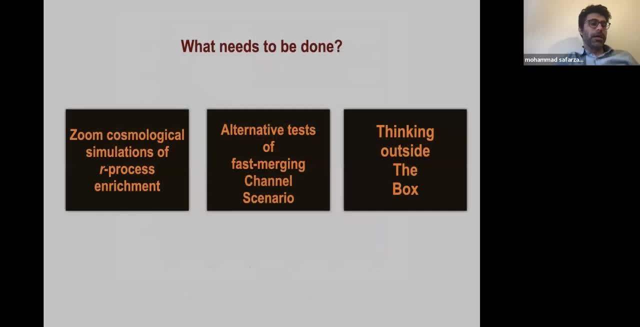 type to make sure that this is a valid argument or not. But what needs to be done? So, other than doing the cosmological simulations of R-process enrichment, OK, OK, One has to come up with other tests of the fast merging channel scenario. 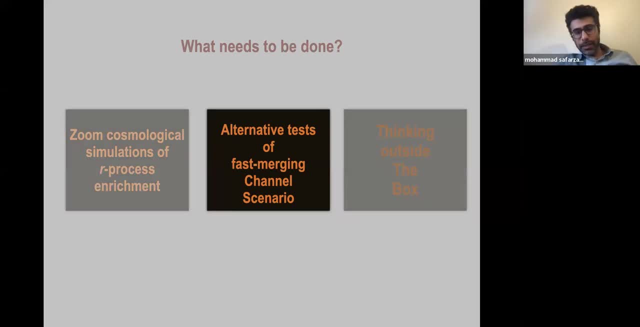 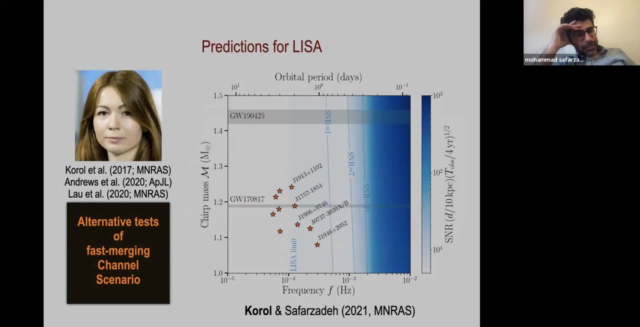 And also sometimes maybe we need to think outside the box. And what do I mean by that? Alternative tests. one paper that we wrote with Valeria Coro is that we said, oh OK, so if this system like 190425,. 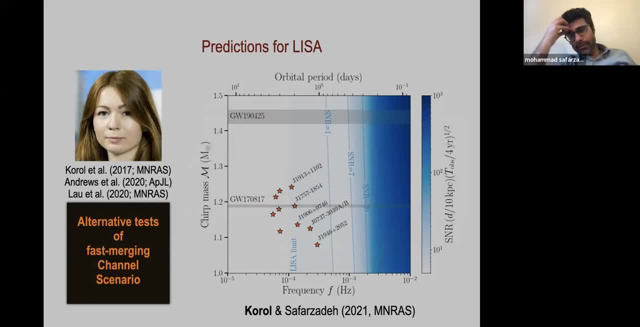 are short binaries, LISA should be able to detect them. So that was interesting. So we said, OK, this system is enough massive that LISA can tell them apart from their less massive counterparts. And then there was a discussion that how long it. 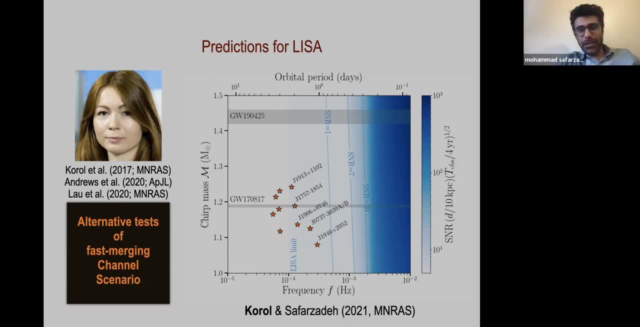 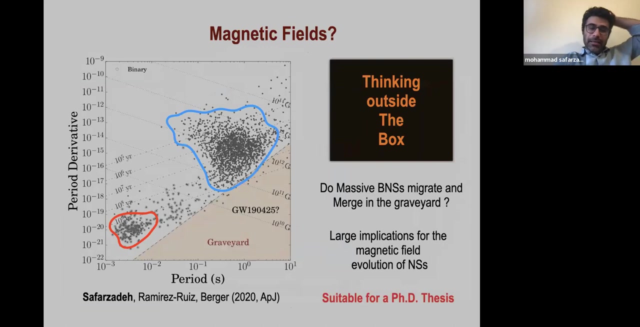 takes for LISA to detect such systems and how far they could be and the implications of that. OK, So for fast-merging channels. So yes, So one can detect them with LISA And that would be very highly interesting. The other idea that we had is that, basically, 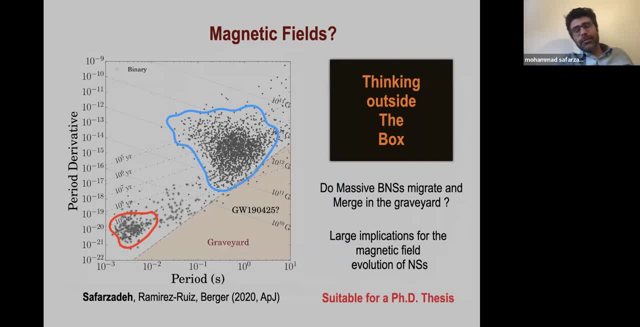 could this be all about electromagnetic waves, Sorry, The magnetic field of a neutron star. And what we mean by that is that if you look at the distribution of neutron stars in period, period derivative, see two blobs: One is for millisecond pulsars in the lower left in the red blob and the normal. 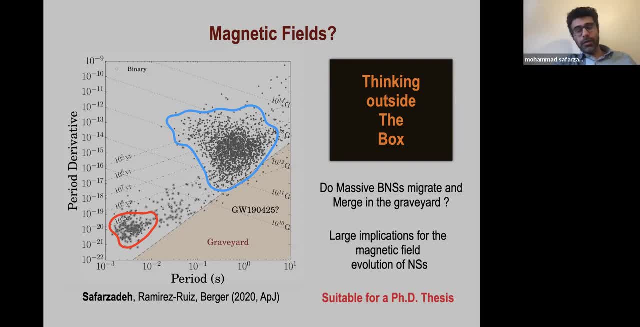 pulsars that are shown with the blue contours. There is a place called graveyard, where the neutron stars spin down and go to the graveyard, and that is where they won't be detectable by radio observations. Now, one idea that we had was: could it be possible that these massive systems 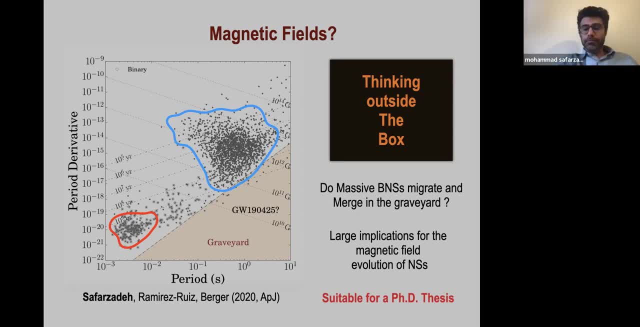 are actually forming, relatively with high efficiencies, similar to the other binary neutron stars that are that we have already observed. but they are. they have migrated into the graveyard. that's why we missed them in radio observations And we can only detect them in gravitational wave. gravitational wave detections. This needs to be modeled in detail. 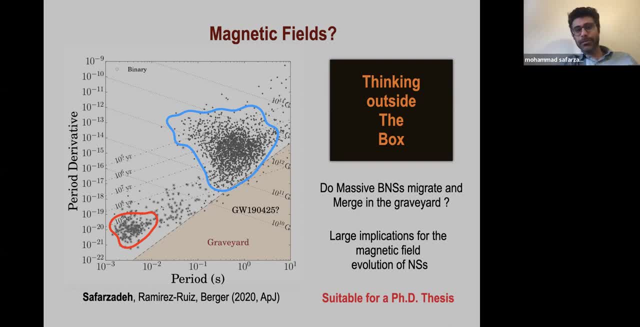 in, basically populations, into this model which is again become perhaps suitable for a PhD project. But that would imply it will have a large implication for magnetic field evolution of massive binary neutrons. So basically, what the theory would be that massive neutron stars are formed such that they quickly migrate to this graveyard. and if this is the case, 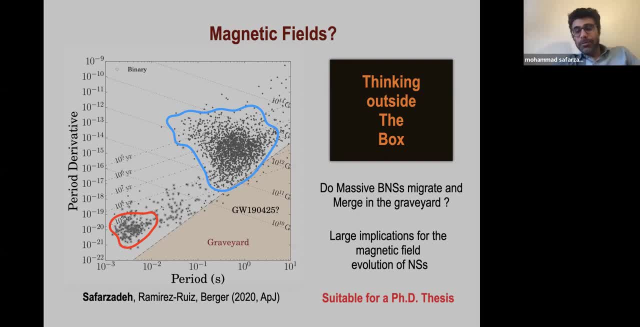 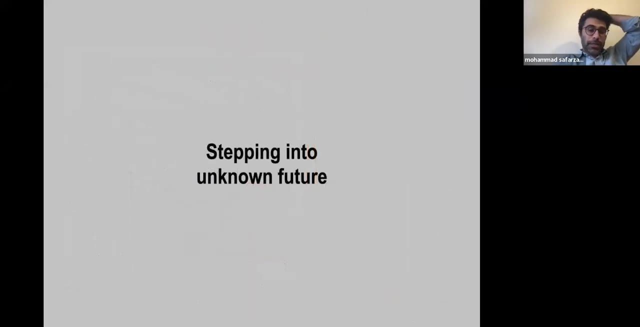 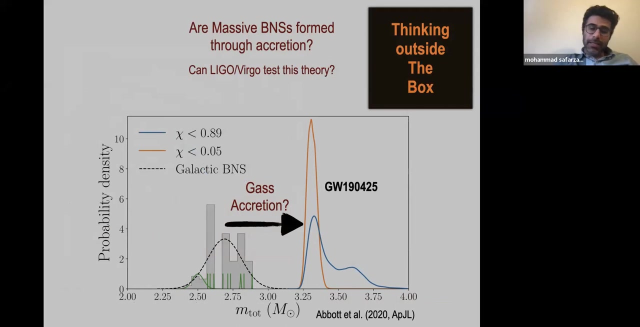 we have a complete bias of the distribution of pulsars in the period-period, derivative and with huge, with large implications. The other scenario that we advocated was that, whether we, whether we could actually detect them in the same way that these systems can form through gas accretion. 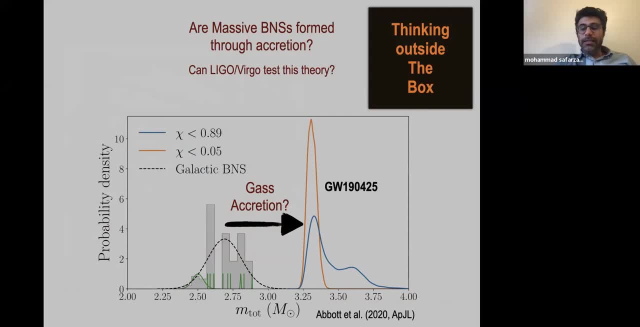 So basically the same scenario that we applied for binary black hole system, but now can this happen for these systems as well? Are these binary? are these systems binary? neutron stars that are that have been accreting gas, for example, in an Aegean disk in a very gaseous environment. they 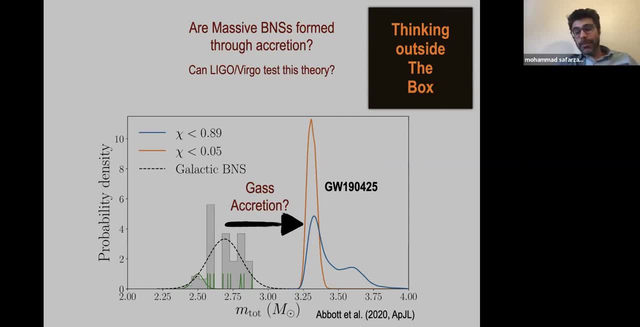 have lived there for a long time. they have been accreting gas. Could it be the case that such a large number of these systems can form in the same way that these systems can form in an Aegean disk in a very gaseous environment? So this is a very interesting question. 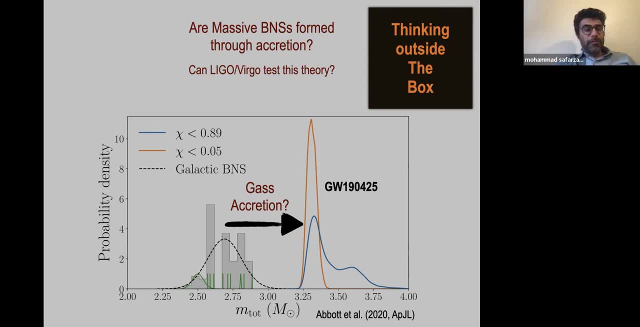 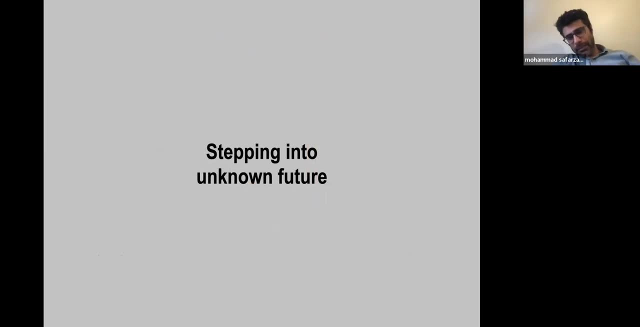 And I think it would be interesting to see how the, the, the environment, is inherently different. This will also have implications for LIGO, but we haven't started working on this one in this scenario yet. So, and to wrap up, I mean we are stepping into unknown field. This is just few examples that I discussed today. Basically, two systems that I discussed today and we will have definitely 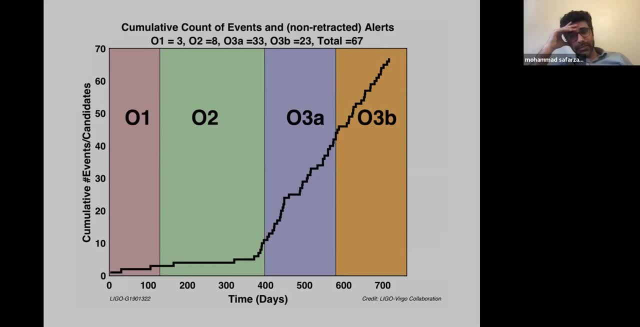 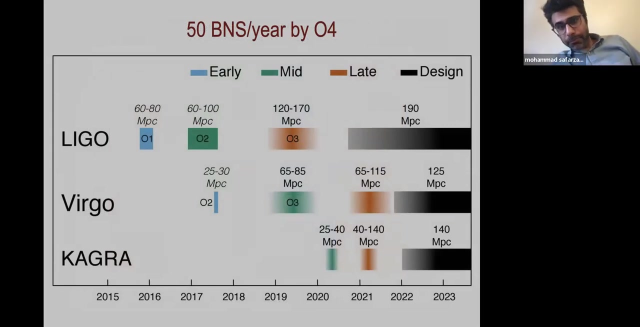 more and more systems. This, the number 67 was, I guess, the number of detections by a few months ago, but now it is more than this and more rare systems have been observed. and it is just the fact that we're going to keep observing about 50 binary neutron stars per year by all four. That's the prediction. 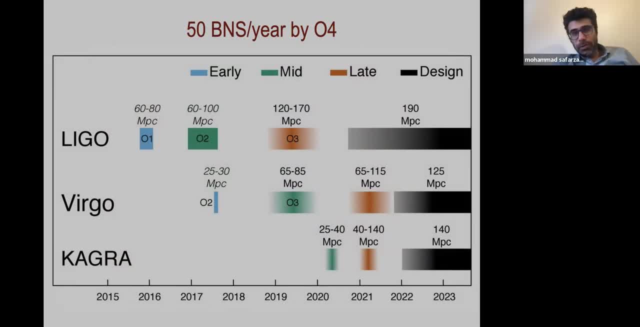 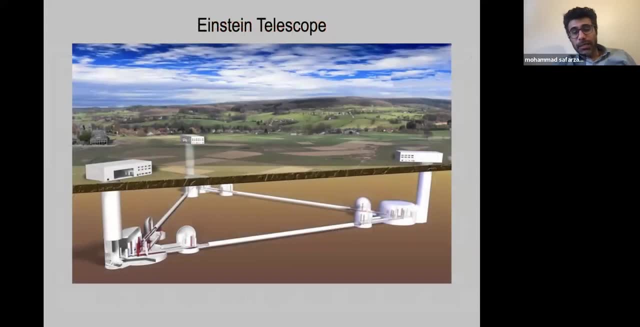 And who knows what we will detect and what will be the mass distribution of binary neutron stars that we would be able to detect by then. And some folks that sit are working on third generation gravitational wave detectors and we know about Einstein telescope and the cosmic explorer that are coming online in the next decade And these systems 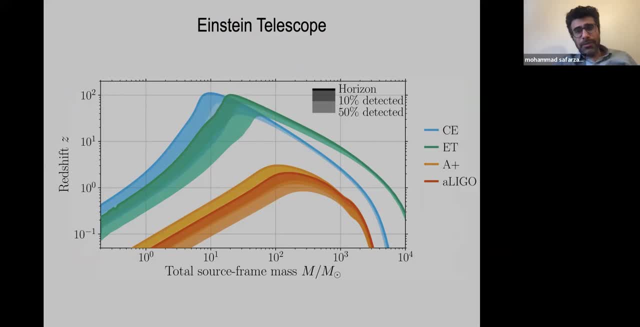 are actually going to see anything that happens in the entire horizon of the universe, And so we will be basically going into 100,000 binary neutron star a year era. But I don't know if we can even have the pipeline for analysis of such observations yet. 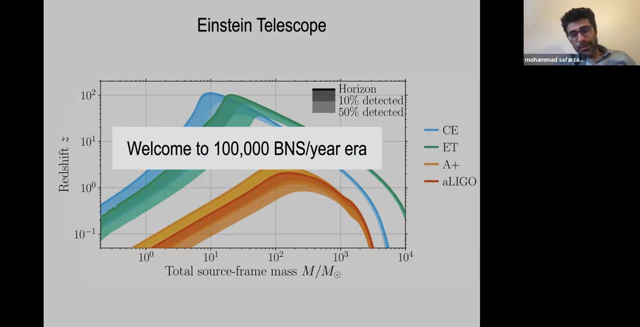 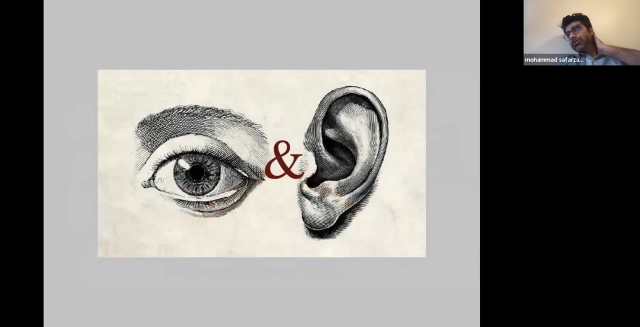 But the discoveries that await us are going to be, of course, revolutionary in nature. So- and this is how much science we could have done only by just two systems- and imagine when we hit this era what kind of science will emerge. I'm eager to see. So at the end, I wanted to just basically 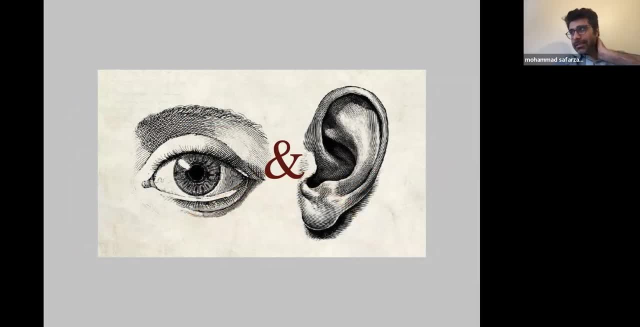 talk a little bit about how different it is like to look at these systems and if you have this mindset of galaxy formation with chemical evolution- and you saw like all of them were relevant, like if you know about the chemicalř evolution, you can have a completely, completely different perspective on the suggested formation. 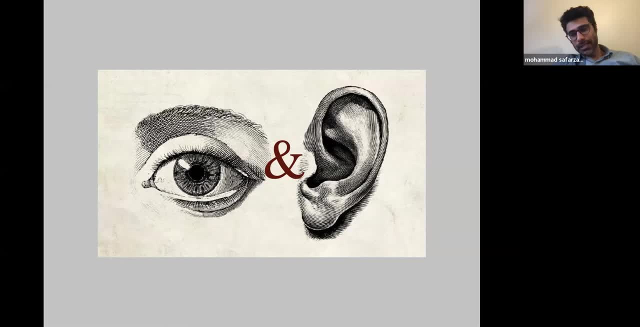 scenarios than if you don't read or think about the the other electromagnetic approaches. so at the end i think that it is always with the combination of these two approaches we can kind of get a correct um interpretation and otherwise we'll get a biased interpretation of this distance. um, i think i stop here and i will take questions, and i hope it was. i didn't. 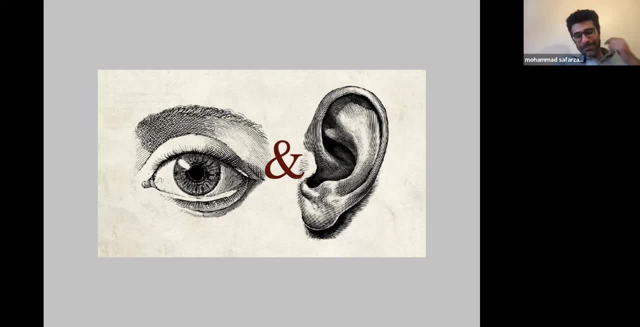 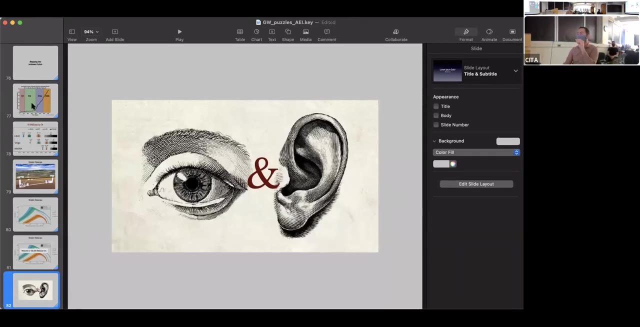 go too fast over some subjects, but uh, ask me if anything wasn't too clear. thank you, perfect, muhammad. thanks very much. very interesting talk. okay, any questions on zoom or in the room? um, uh, norm, do you have a question? yeah, i was gonna ask about you. you sort of quickly mentioned. 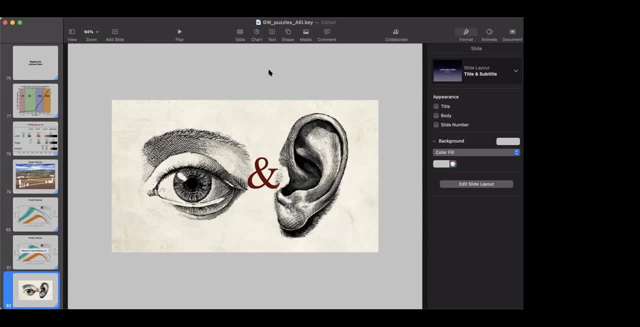 accretion onto both binary black holes and binary neutron stars. uh and, and there was also some you know sort of time involved there- you wanted to double their masses. so that would be my recollection is: double your mass on a black hole at Eddington. 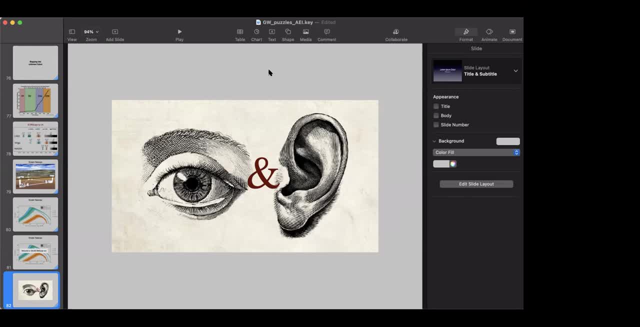 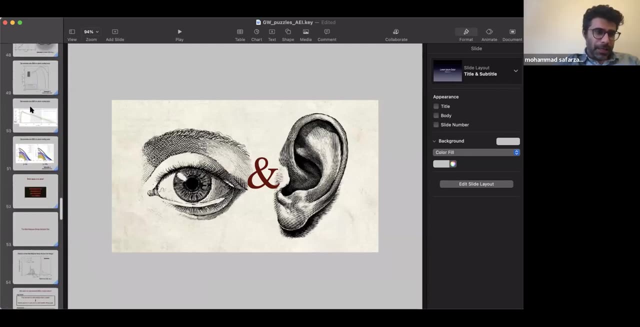 would take something like 50 million years. That's not any kind of sort of delay time, but what you know. so I want to get a feeling for the accretion rates that you're looking for, Right? so what did this? let me bring up the slide. 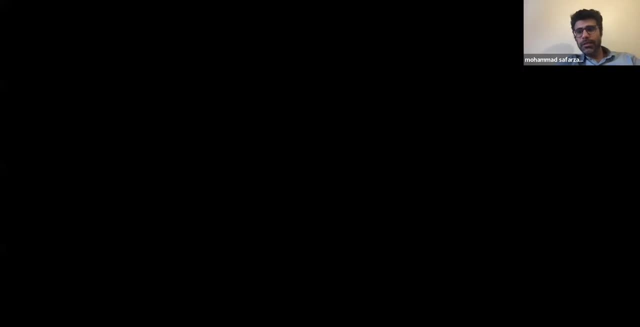 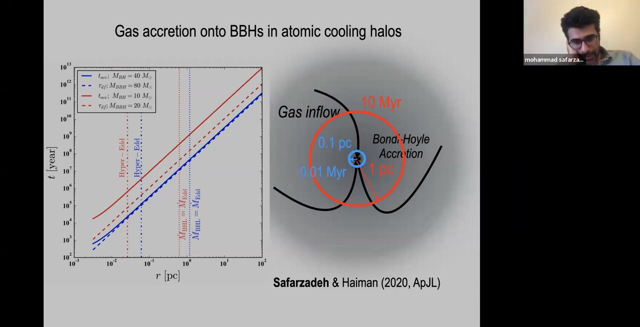 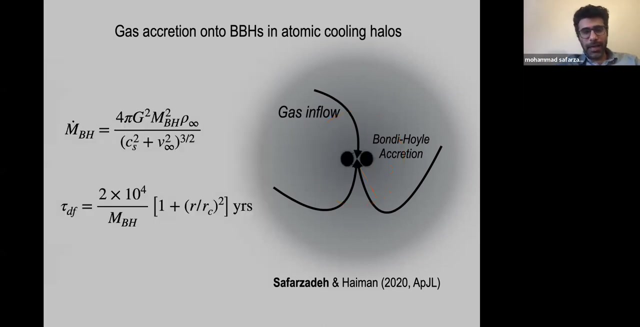 maybe this. so the left panel of this plot shows how long it takes for the binary black hole to double its mass, and different lines are showing for different masses of the binaries. And it depends on the mass of the binary because of course the m dots just itself depends. 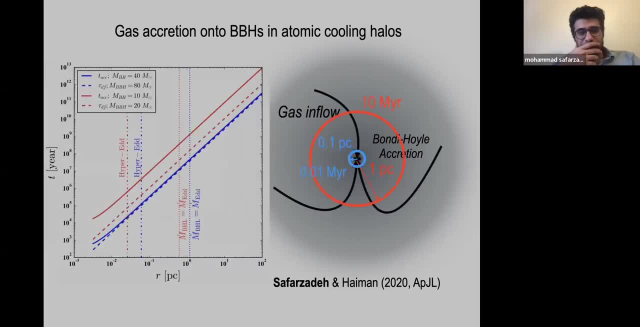 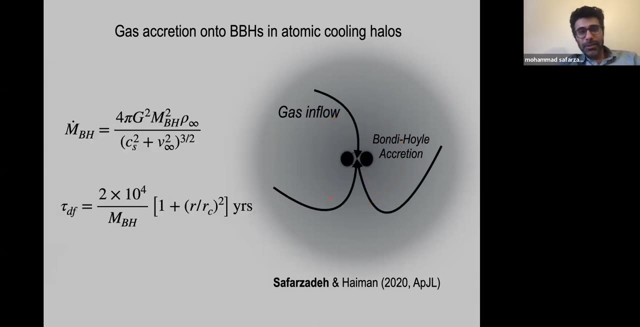 on the mass of the binary square. But what we did is that we are assuming also the here, the m dot that we are getting is also depends on the environment that we are. So for the calculations that we did, the mass accretion rate was the function of radius. 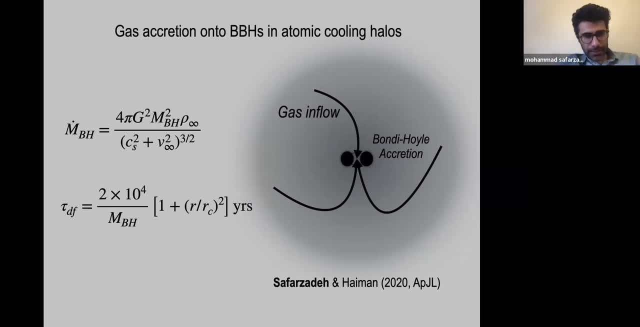 from the core of the atom, And we did that on a cooling halo, because that sets the density and also its temperature, was setting the sound of speed after medium And for so that's how we computed the mass accretion rate And we compared the time for doubling the mass compared. 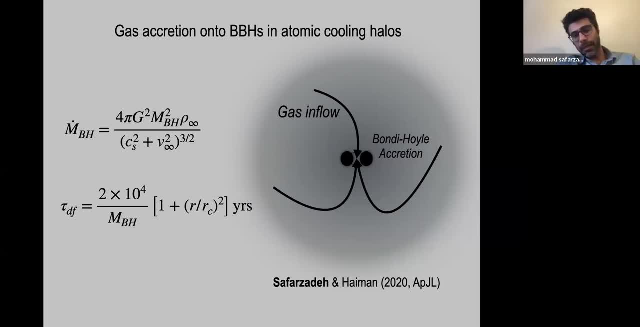 and we compared that to the dynamical friction of the system, which depended on where is this black hole rotated and how far it is from the the center of the atomic cooling halo. So we basically tried to compare these two and say that 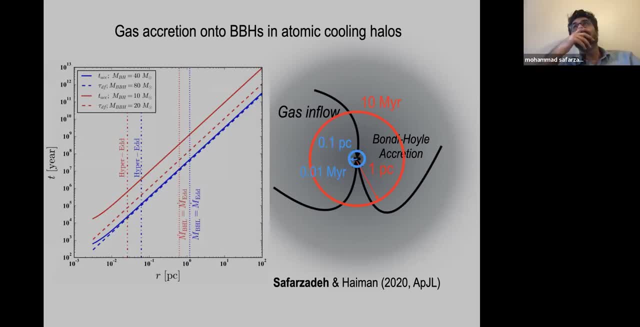 oh, okay, so if the time to doubling is less than the dynamical friction time, then this is an acceptable theory, And then what we find is that they're almost the same time scale. One issue with doubling the mass that I was referring to. 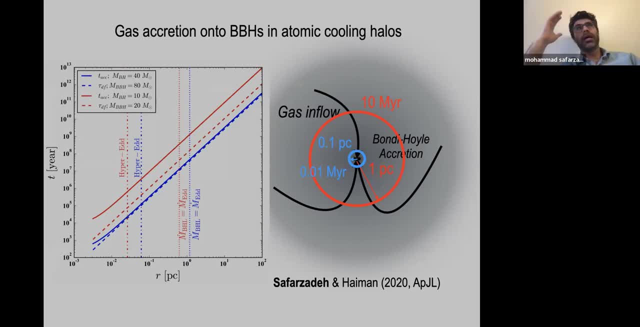 is that the idea is that by the time you double your mass, you have to merge because- or in other words, people are arguing is that you can never accrete more than you cannot triple your mass before merge. If you double your mass, you couldn't merge. 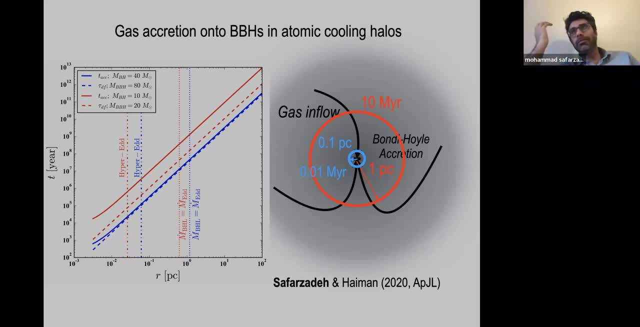 So basically, this is the theory, But I don't believe in that because this is very simplistic derivation in the sense that what happens to the gas when the binary black hole is in very, very short distance is problematic in the sense that prior to 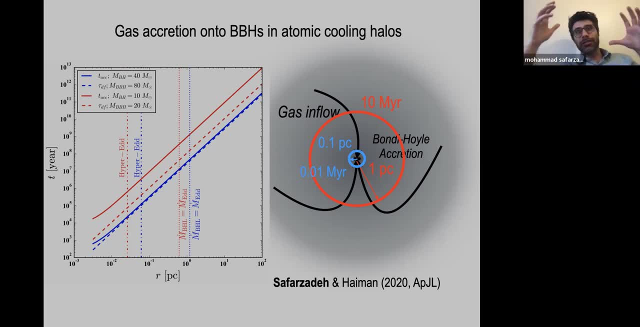 at large separations. yes, you can accrete, and this accretion is gonna take away the angular momentum of the binary, and then you shrink further and further while you're increasing your mass. But it is not clear that this is the case. 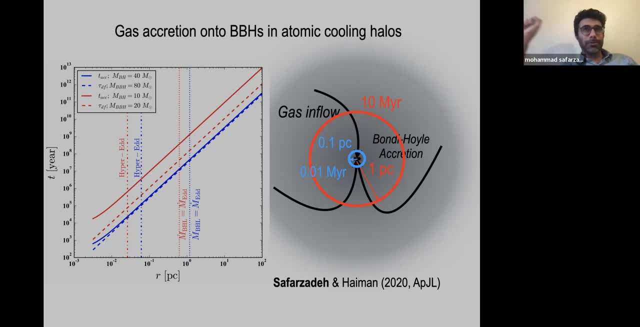 It is not clear that this process is all the way through, all the way to the merger, because at very short separations the orbital velocity is gonna go supersonic And now the gas that re-heats the binary is gonna get shock heated. To me it's not clear that it's gonna take away. 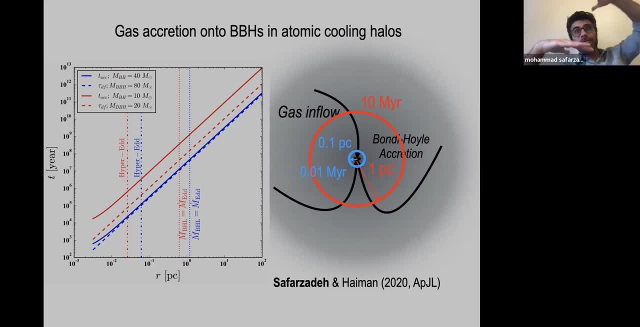 the angular momentum anymore And perhaps you can accrete from different directions and still you increase your mass, but you do not necessarily. also, the gas accretion does not necessarily lead you to merging. but this needs hydrodynamical simulation like very detailed hydrodynamical 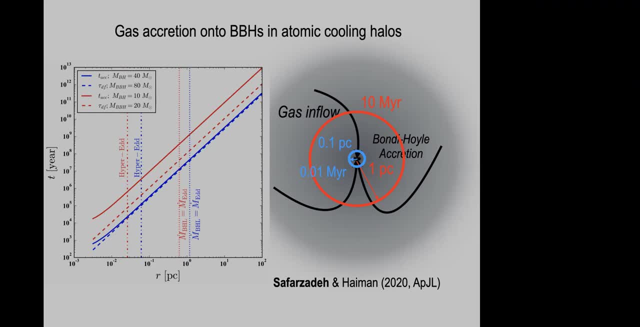 Well, I had an even simpler worry was if you're creating at anything. right, There's a lot of feedback on the gas and Bonnie isn't gonna work. That's the amount of accretion. So when I was writing this paper, 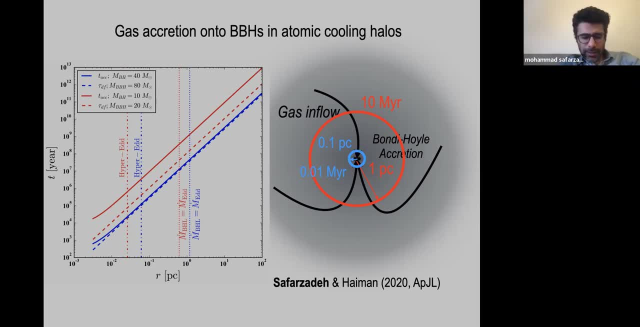 I read a lot about this, And so what I'm understanding is that the it is divided. So there is a feedback that you have and you're gonna stop that accretion, But again it's like a phase that you have to wait in. 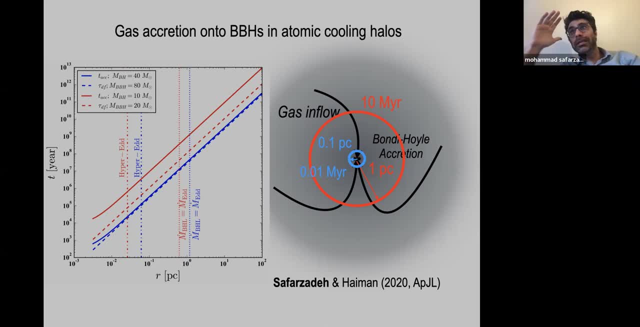 and then it can also be overcome. So if you go to, if the accretion rate is about 500 Eddington, then you can just accrete again with no problem, as the photon itself is gonna be also accreted. The whole energy density is gonna be accreted. 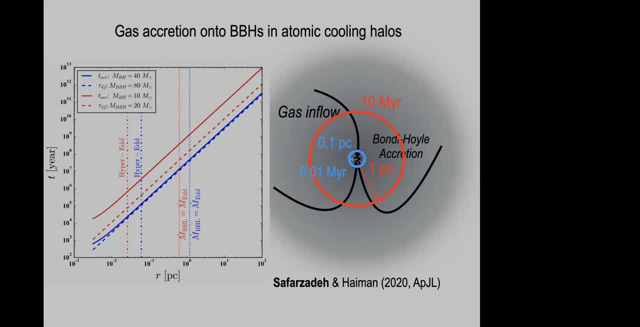 And then the system. So I agree with that. But I mean, so you're arguing that you're sitting in the center of some halo and accreting. is that the idea? Cause if you're just in it, most of these stars are gonna form in. 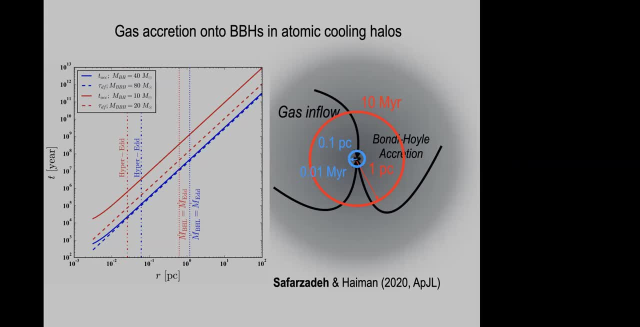 are these you're talking about in dwarf galaxies? What kind of galaxies is this things forming in? Yes, So these are binary black holes from population three year stars that have been forming at super high redshift, And the idea is that, yes, there are papers. 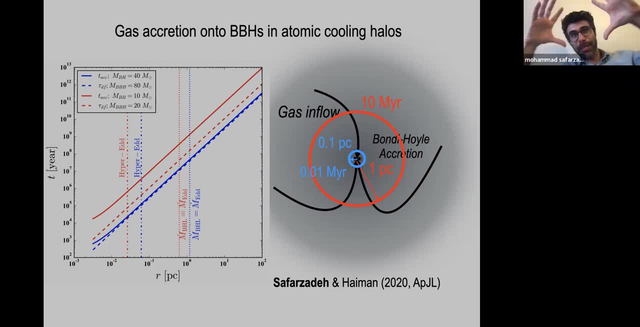 that showed that including and not including the feedback is gonna really impact the how much mass we can accrete. Accrete, yeah, Okay, but you're imagining that they're sitting at the center of the halo. That's really the point here. 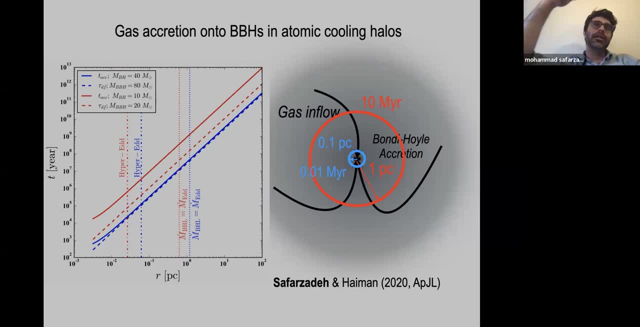 We are saying it is migrating around, the halo around, and then it is gonna dynamical friction due to dynamic Fall into the center, Yeah, okay. But we are saying that it can. it can go to accretion rates above hundreds of Eddington. 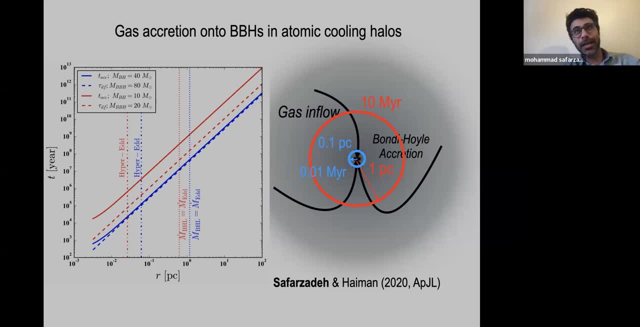 because these systems are extremely dense at high redshift- The atomic cooling halos. that was like a part of the argument and not the whole part of it, but that was the contributing part of the theory that you can actually overcome this issue. And another thing that I wanted to add is that 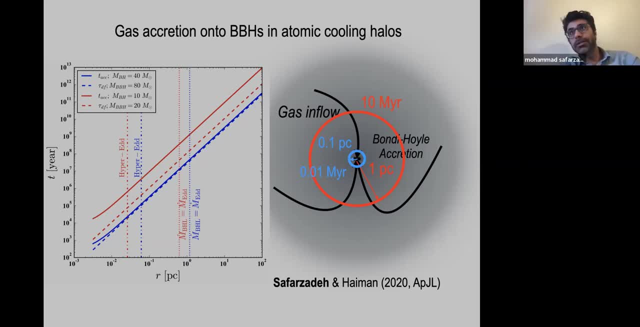 these simulations are already done, These simulations of accretion of gas into seed black holes are already done, with the aim to explain the quasars, million solar mass, quasars at high redshift. And here we have even a much simpler ask. 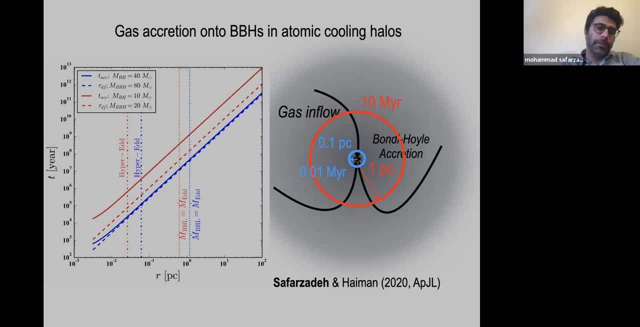 We don't wanna increase them to millions of solar mass, We just wanna double their mass. That's all I wanna do. So to us that should be easier, much, much easier. And so if people have been trying and people have been writing about it, 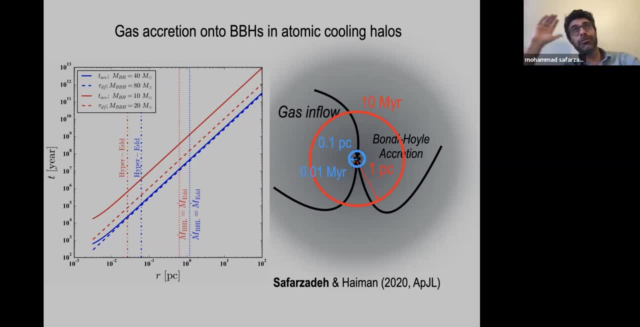 even like since 2006 that, oh, if you turn on the accretion you're not gonna make seeds for quasars at high redshift. But this is not what we want here. We don't wanna increase them to millions of solar mass. 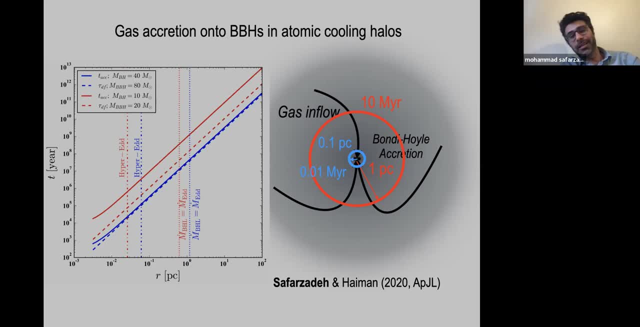 We just wanna double the mass. Can we do it? It doesn't seem too difficult, And the beauty of this is that you don't necessarily need to fine tune this, And it is also possible that you relax the binaryness of it and just grow each one. 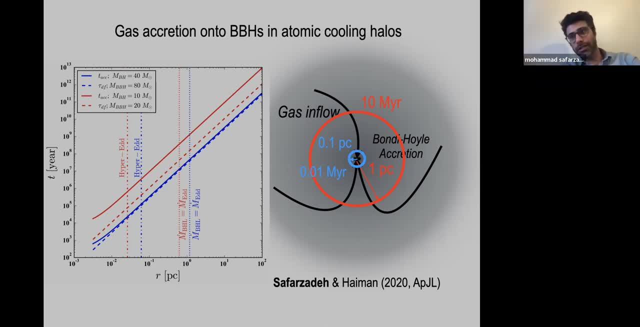 of them individually and then merge them together later on. So you can actually accrete to two individual halo black holes in atomic cooling halos and then bring them together dynamically and merge them. That is possible, That is plausible, But- and some people like that scenario better- 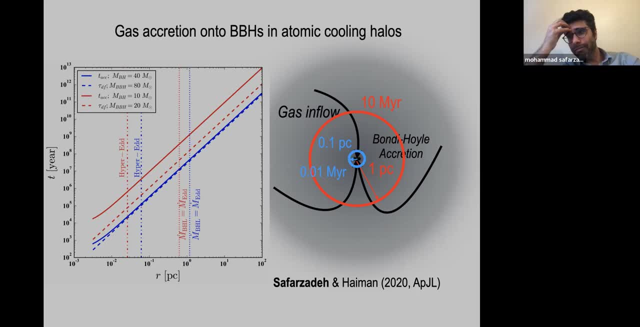 but I'm not sure how fine tuning, how much fine tuning would be involved in that scenario. But to me this increasing or doubling the mass before the merging doesn't seem to fine tune of a scenario if you adapt it through gas accretion. 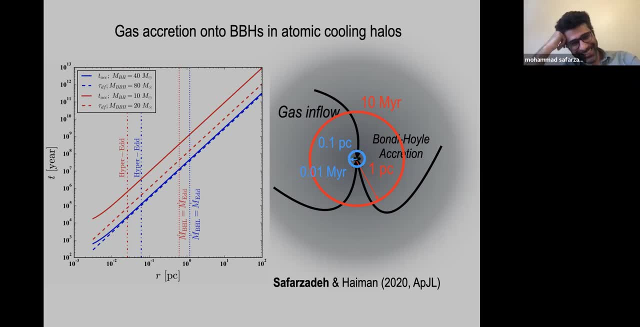 in atomic cooling halos. This is a short answer. Thanks, Mohammad. Was there another question from Chris? Do you still have your hand up? I was mainly going to ask the same thing about feedback, I guess, when it comes to photon feedback. 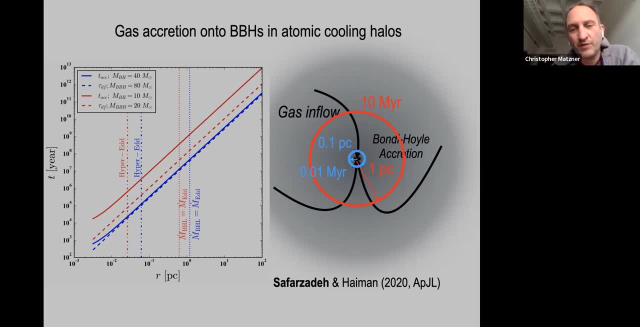 you can overwhelm it, But there are these. if you add magnetic fields to the mix, it can become more complicated, as I understand, And so you can get inflow, outflow solutions and also energy extraction directly from the black holes. So it's not obvious. 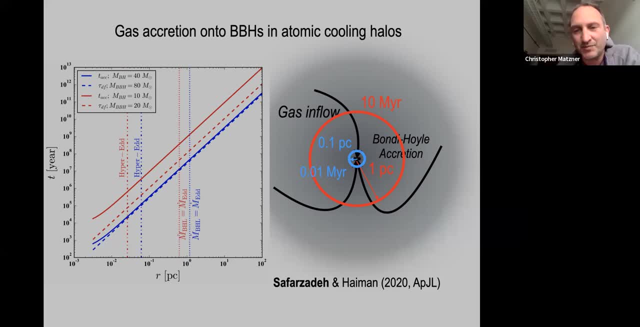 It's not obvious, So you can just dump material onto them. But I think also, when it comes to accreting material, even if you ignore feedback, it makes a big difference whether the gas you're trying to accrete is rotationally supported, has more angular momentum. 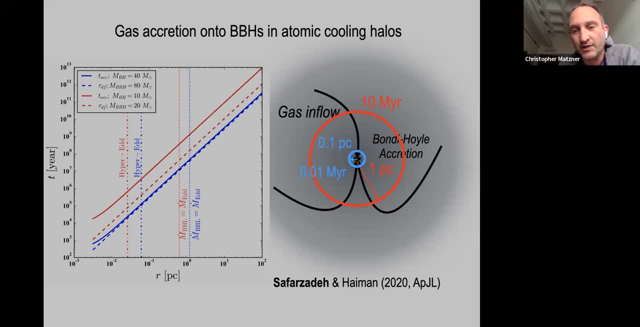 than the binary, or not. So if it does, then you're doing gas accretion through a disk and it's like binary star formation, which doesn't doesn't necessarily have to shrink your vitamin. ah, okay, that's a good point. yes, yes, 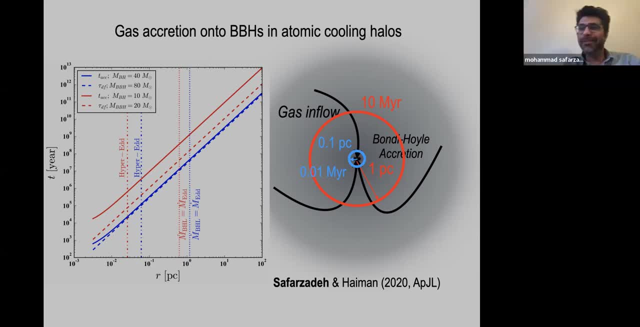 that wasn't really a question there. yeah, no, thank you for the comment. any any last questions on zoom or in the room? if not, let me sneak one quick one. in muhammad, at the beginning, you uh gave a- just you know, a simple estimate, a rough estimate, maybe 300 binary. 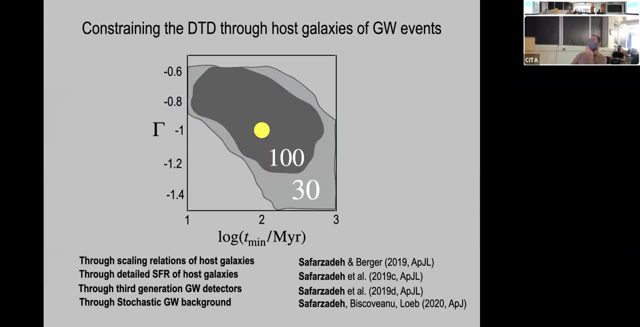 neutron stars with em counterparts in order to distinguish the fraction- yeah exactly, you know- of field formation versus dynamic dynamical formation. i'm just wondering: is 300 a little bit pessimistic? because can you not do some sort of statistical association between you know the sky localization? 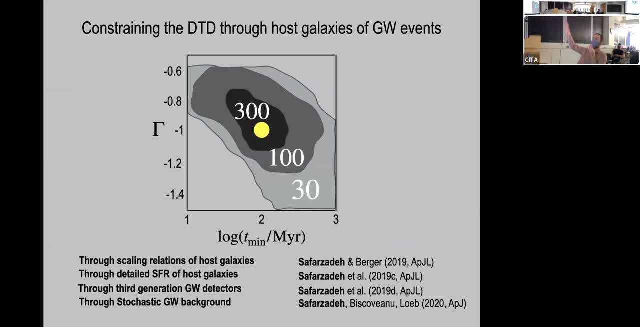 the distance measurement and the host galaxy. does that sort of thing buy you anything? do you really need the em counterpart in all cases? uh, so the uh. so we wrote a paper, different paper, that just used the, the scaling relation of the host galaxies, and we got about the same answer. so, any, any way, i tried it. it's very pessimistic. i wrote four. 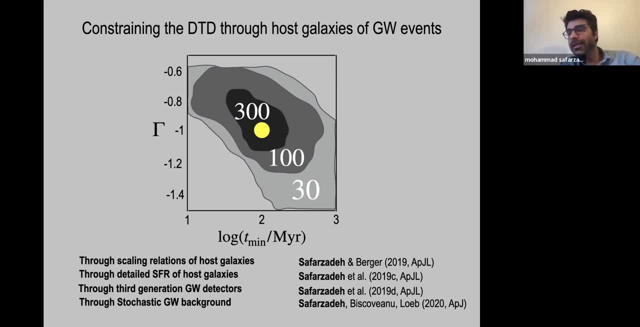 papers in this, and even with third generation, is extremely- oh, i wasn't getting really good results. i mean, okay, third generation gravitational wave detectors. of course you can do a lot to them, but even then you need like a year-long observation to pin down different, uh, different formation, um, different delay time distributions, because, again, the 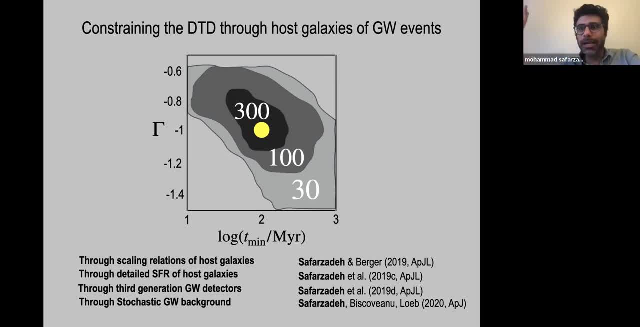 the error on the redshift of the source, although you detect them at high ratchet, but the error bar on the redshift is going to also explode with redshift. so you, so you need a lot of observation, integration, integration time for third generations to actually even do this by them, by them. so whether 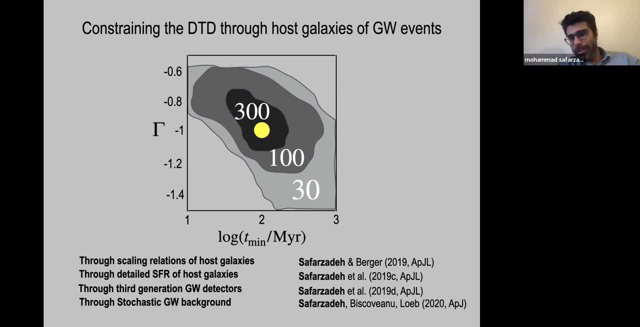 you can add more information to this. perhaps you can add more information. you mentioned the sky localization. is that what you? you're saying that there's extra piece of information? 3d localization- yeah, 3d localization, statistically associating it with the horse, the host galaxies that are in that. 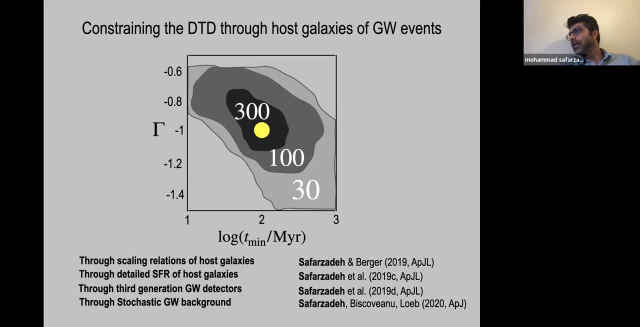 uh, you know area, so so So are you worried about the kicks? Is that what you're worried about, So that the kicks are gonna? no, Are you talking about just like, basically, two point correlation function of this distribution? That's exactly, that's all I'm saying.